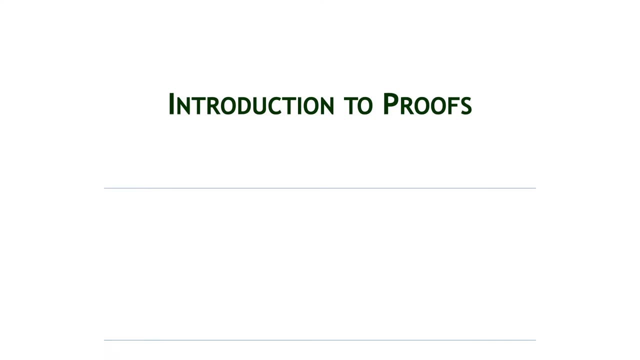 Hi everyone. In this video we are going to talk about introduction to proofs. First we are going to give a brief introduction, Then we are going to study some of the methods that are available for proving theorems. We are also going to see some mistakes that we can make. 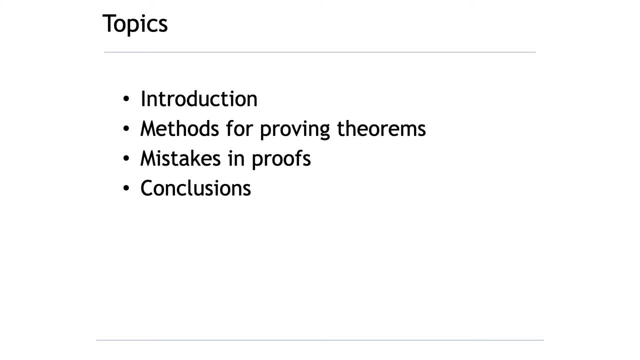 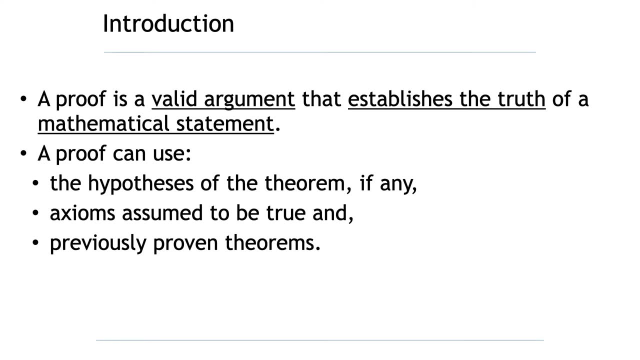 in proofs And finally we are going to state the conclusions. A proof is a valid argument that establishes the truth of a mathematical statement. Notice that from previous videos we already know what is a valid argument. We also know what. what is the truth? value of the. 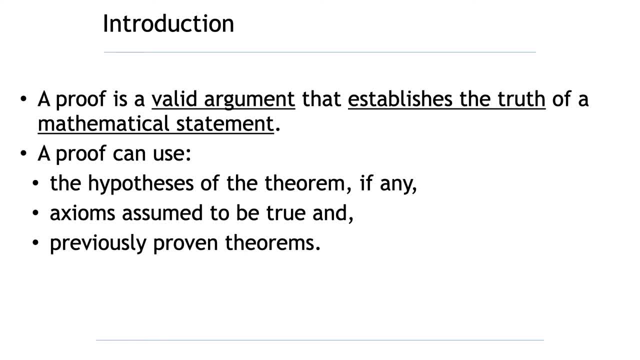 mathematical statement. If you didn't watch those videos, I'm going to leave the link below, So please watch them before you move forward with this topic. A proof can use the hypothesis of a theorem. It can also be used to prove a hypothesis of a theorem. 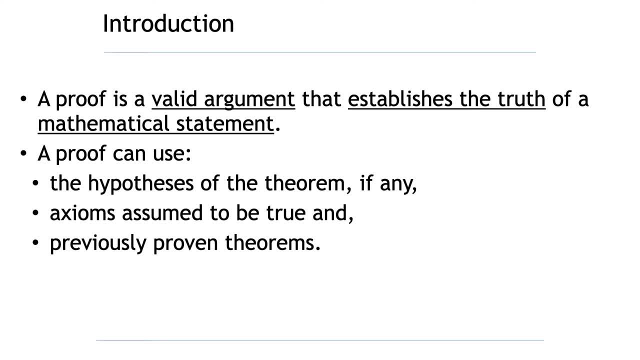 A proof can use the hypothesis of a theorem. It can also be used to prove a hypothesis of a theorem, If there is any. it can also use axioms assumed to be true and previously proven theorems. Using these ingredients and rules of inference, the final step of the proof establishes the truth. 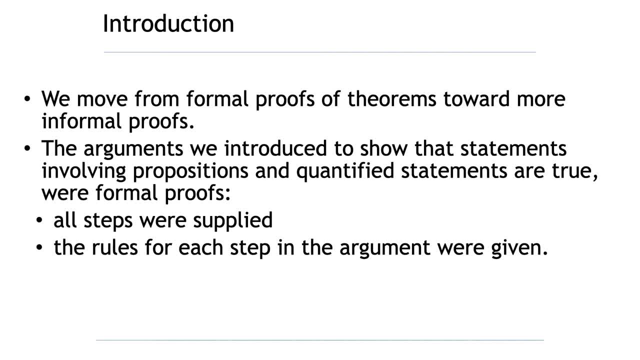 of the statement being proved. We are now moving from formal proofs of theorems toward more informal proofs, As in previous videos, we saw that in each proof we need to supply, we need to show every single step and we need to justify every step with the rules that we are using. 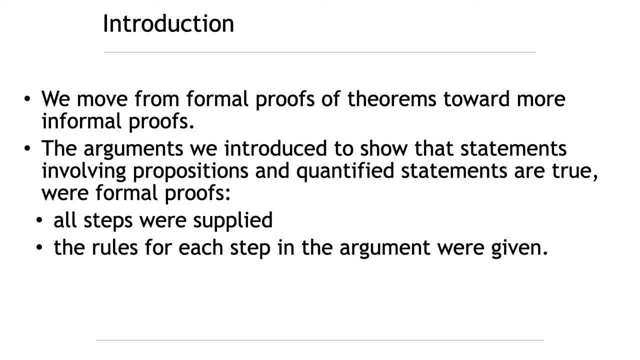 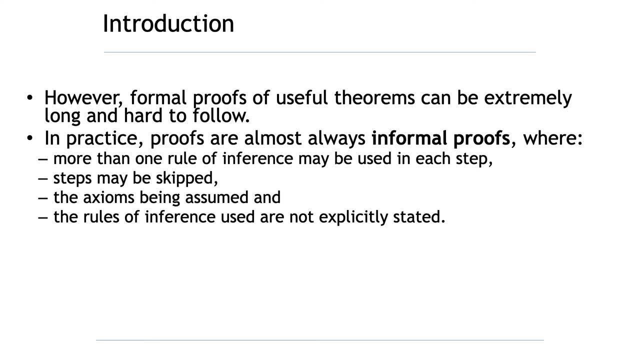 So in this case now we are going to move towards more informal proofs, and you will see what is the meaning of that during this video. So formal proofs of useful theorems can be extremely long and hard to follow In practice. these proofs are almost always informal proofs. In these informal proofs, sometimes more than one rule. 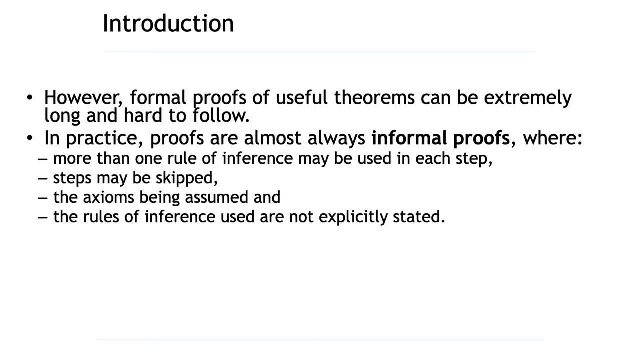 of inference is used in each step. Some steps may be skipped. The axioms being assumed and the rules of inference used are not explicitly stated. This doesn't mean that you can do it in any way you want, For instance, if you say that you want to do something in a certain way. For example, if you say that you want to do something in a certain way. 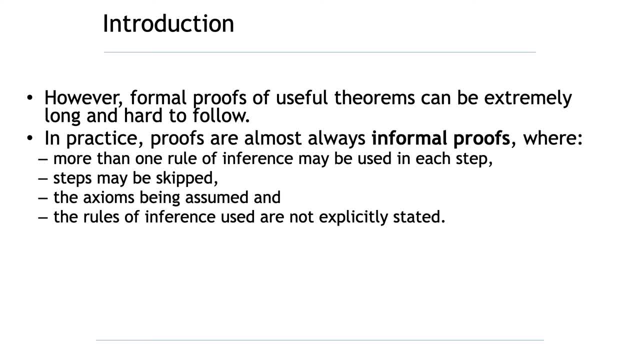 you skip one step. that step must be obvious for the reader. Informal proofs can often explain to humans why theorems are true, while computers are perfectly happy producing formal proofs using automated reasoning systems. Obviously, the computer cannot make an informal proof. 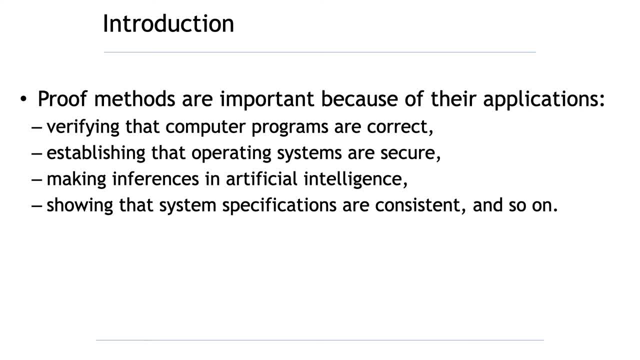 Proof methods are important because of their applications. They can be used to prove that the proof is correct and they can be used to prove that the proof is false. be used to verify that the computer program is correct, to establish that an operating system is secure. to make inferences in artificial intelligence, to 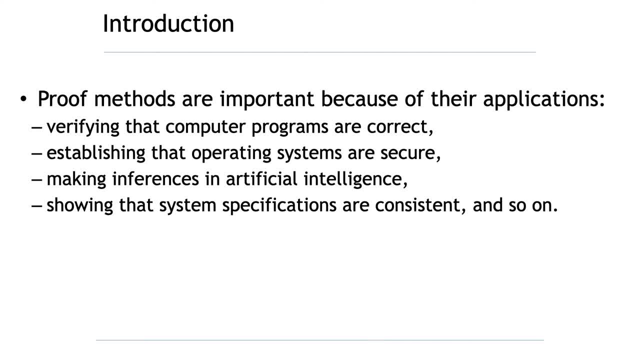 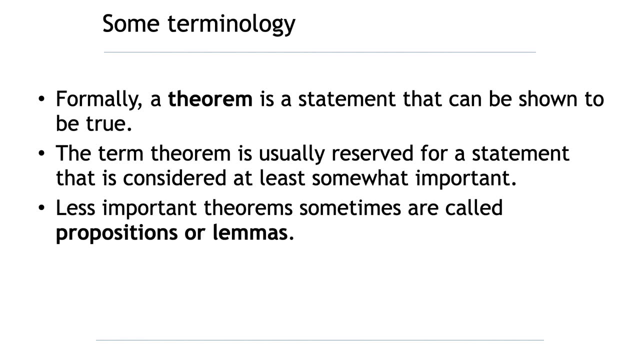 show that system specifications are consistent, and many other. Therefore, understanding the techniques used in proofs is essential, both in mathematics and in computer science. So now we start with some terminology. Formally, a theorem is a statement that can be shown to be true. The term theorem is usually 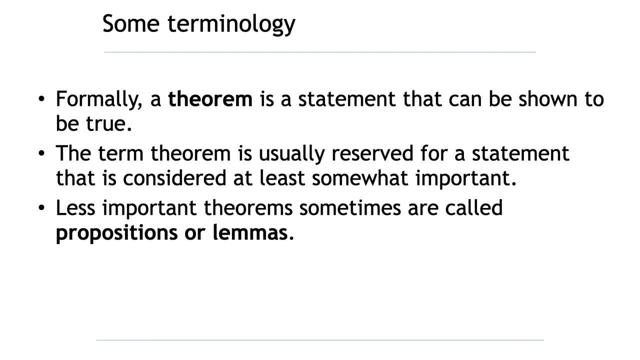 reserved for a statement that is considered to be somewhat important. Less important theorems sometimes are called propositions or lemmas. Theorems can also be referred to as facts of truth. Remember that I mentioned in previous videos how important are definitions in mathematics. If you see from the definition of a 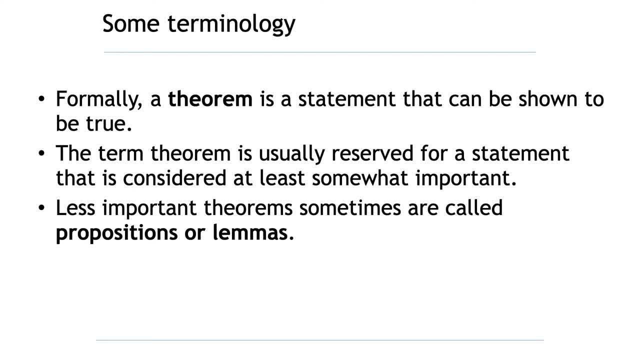 theorem. it is a statement that can be shown to be true. What does it mean? It means that if it is not true, then it's not the theorem. Here we cannot apply the same than propositions. OK, Remember, propositions are statements. 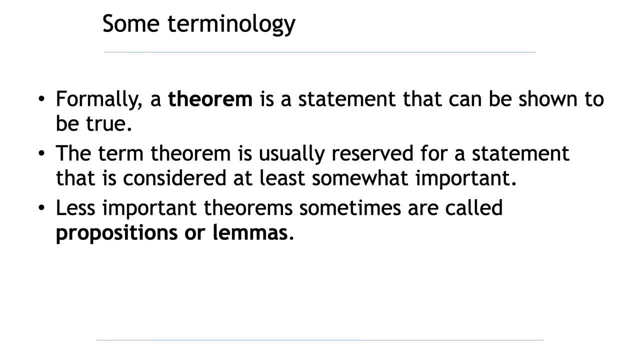 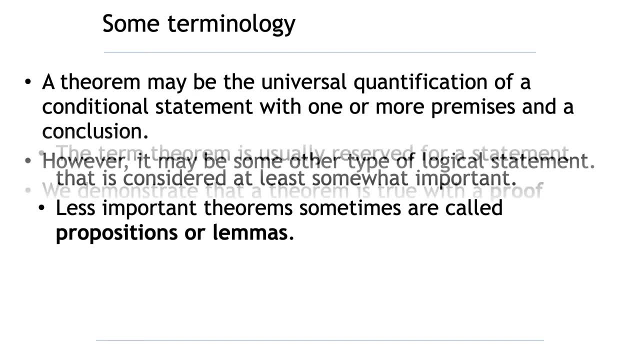 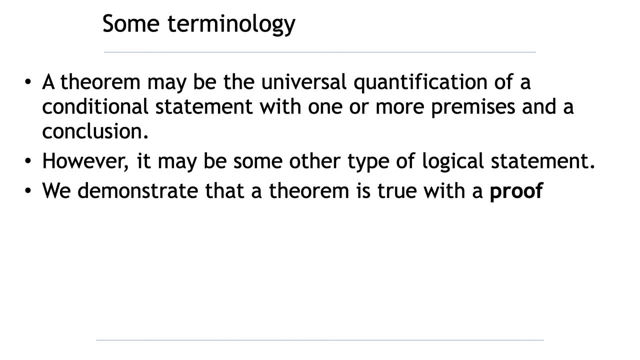 that can be true or false. In the case of a theorem, it has to be true. It cannot be false. A theorem may be the universal quantification of a conditional statement. These statements can have one premise or more and it always has a conclusion. 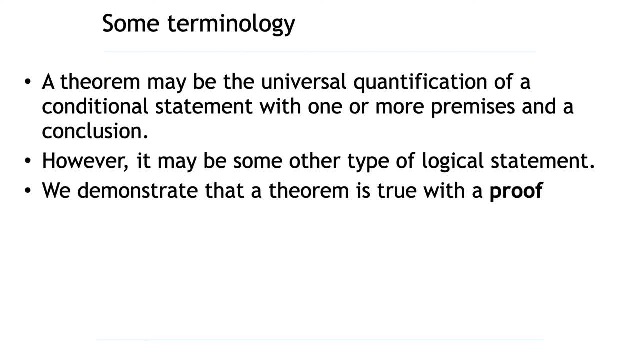 However, it may be some other type of logical statement. The way that we demonstrate that the theorem is true is with a proof. Remember, we already saw how to create formal proofs. In this case, we are going to move toward more informal proofs. 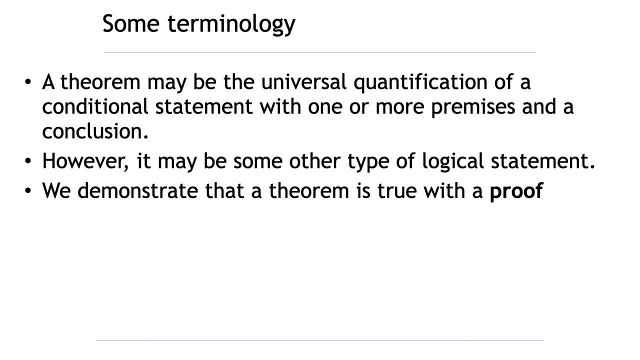 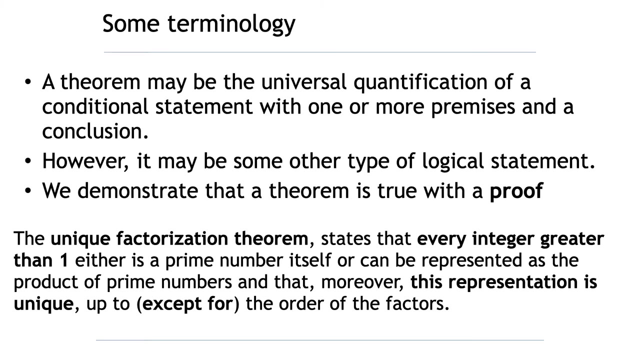 It doesn't mean it is just an informal proof. As I explained before, it has some rules. The reader needs to find it. It's obvious, the steps that are being skipped, and so on. A theorem may be the universal quantification of a conditional statement. 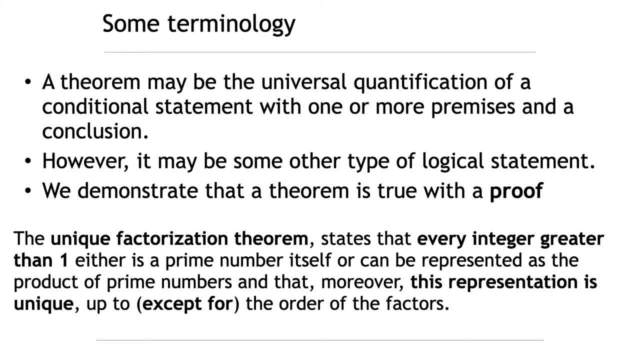 with one or more premises and a conclusion, as I mentioned before. So let's see this example of a theorem. A theorem states that every integer greater than one either is a prime number itself or can be represented as a product of prime numbers. 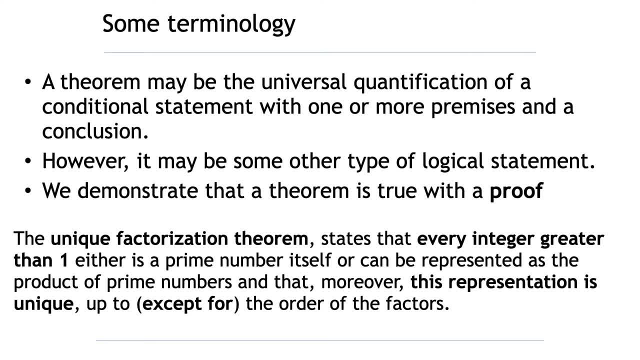 and that, moreover, this representation is unique up to or except for the order of the factors. What do we have here? We have here several premises and we have a conclusion. What is the conclusion? in our case, The conclusion is that the number, it is prime number itself. 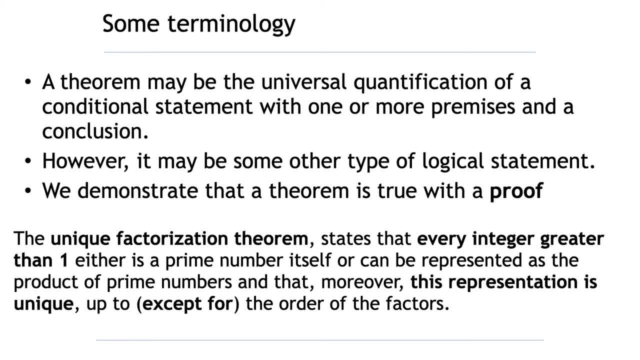 or it can be represented as a product of prime numbers. okay, And then the premises in our case is that the number is integer and is greater than one. So in this case we have two premises. This is an example of a common theorem. 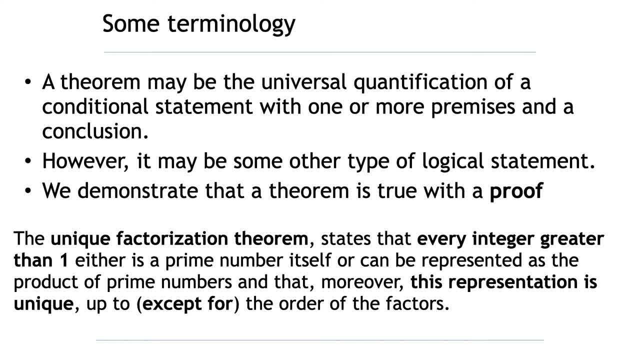 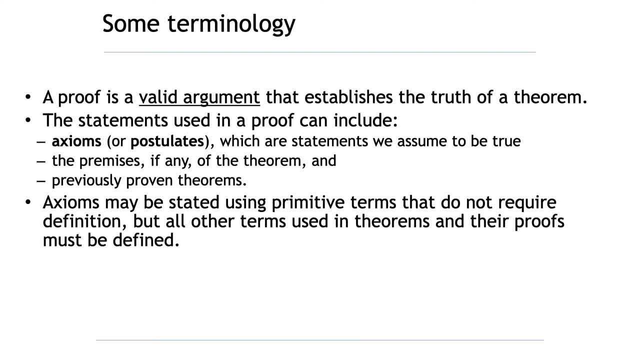 and through this video series you will see more of them. A proof is a valid argument that establishes the truth of a theorem. We already know what is a valid argument and in previous videos we made some proofs, So the statements used in a proof can include axioms, which are statements we assume to be true. 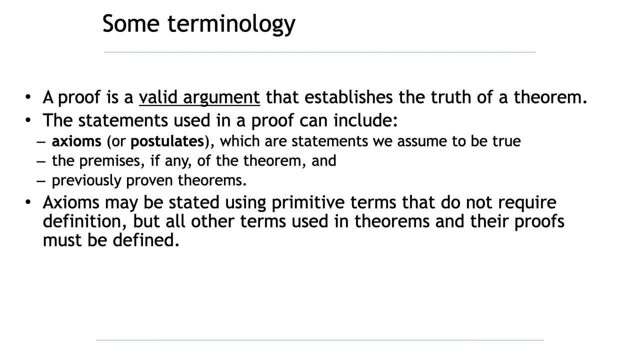 and we don't need to prove them. the premises: there are premises and previously proven theorems. Axioms may be stated using primitive terms that do not require definition, but all other terms that we are going to use in a theorem and the proofs must be defined. 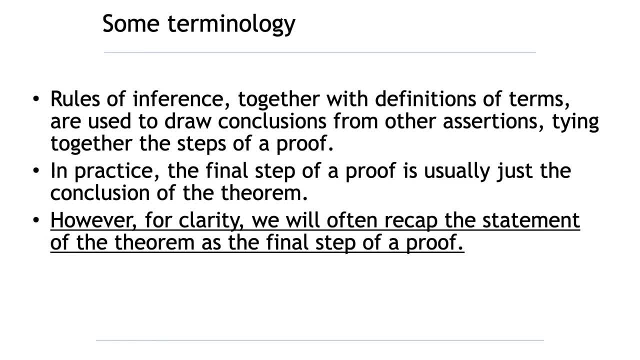 Rules of inference, together with definitions of terms, are used to draw conclusions from other assertions tying together the steps of a proof. In practice, the final step of a proof is usually just a conclusion of the theorem. However, every time we create a proof of a theorem as the last step, 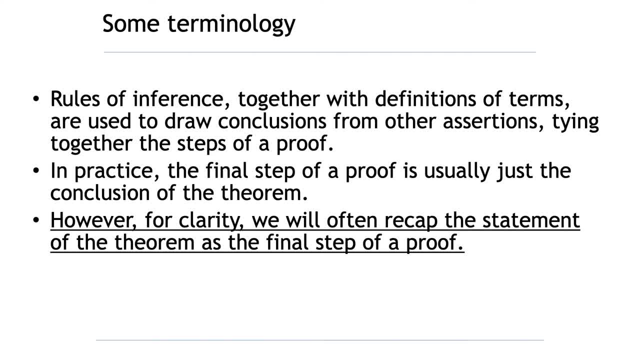 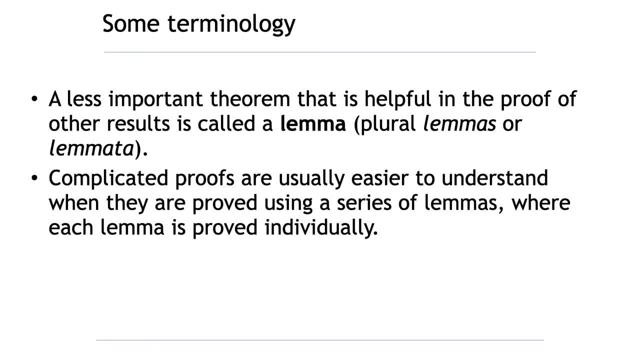 we are going to recap the statement of the theorem, So we make more clear the point that we want to prove. A less important theorem that is helpful in the proof of other results is called a lemma. Usually complicated proofs get easier to understand when they are proved using a series of lemmas. 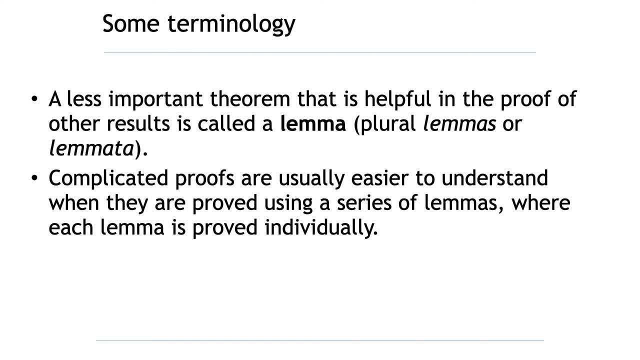 where each lemma is proved individually. This technique is a similar technique used in algorithm design. that is called divide and conquer. So in this case we are just trying to divide the big theorem, the big complex theorem, in smaller parts so that we can prove those smaller parts individually. 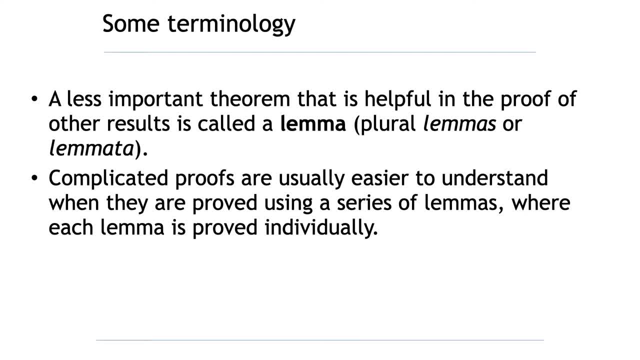 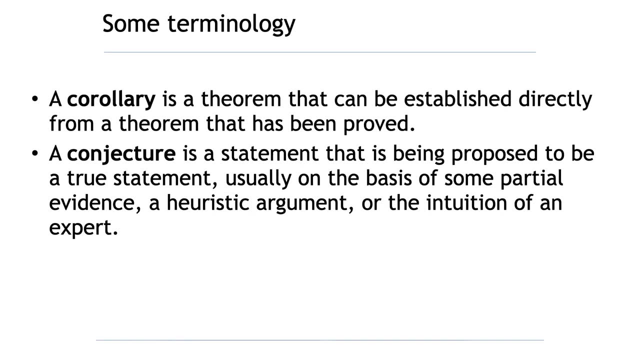 After we prove the individual parts, we use those partial results to prove the theorem. That makes our proof more understandable and easier to read for everyone. A corollary is a theorem that can be established directly from a theorem that has been proved. Sometimes you prove a theorem that generalizes a certain conclusion. 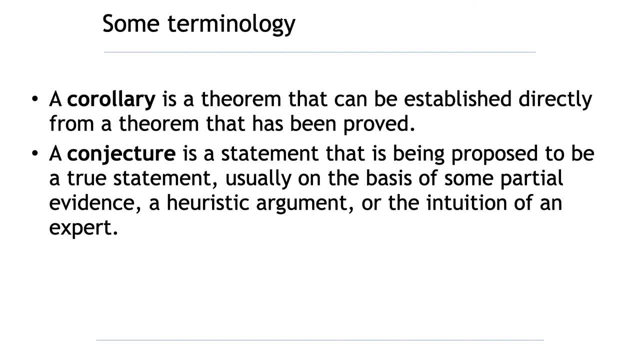 but it can be useful to have a theorem for a specific case of the general theorem. That can be written as a corollary and because it is a specific or special case of a theorem that has already been proven, it doesn't need a proof. 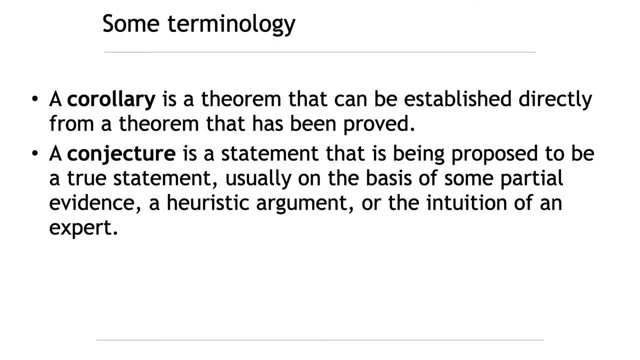 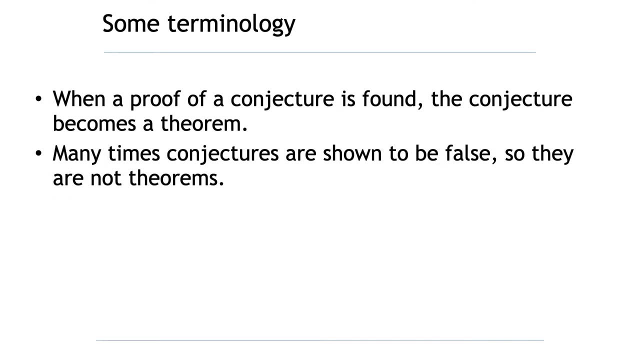 A conjecture is a statement that is being proposed to be a true statement. used to prove a theory, Usually on the basis of some partial evidence, a heuristic argument or the intuition of an expert, but it is still not being proved. When a proof of a conjecture is found, the conjecture becomes a theorem. 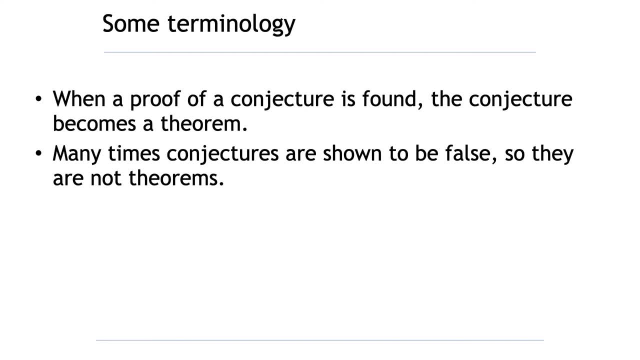 Many times, conjectures are shown to be false, so they are not theorems. So remember- this is a very important point- Theorems are always true. Theorems are always true. Theorems are always true. 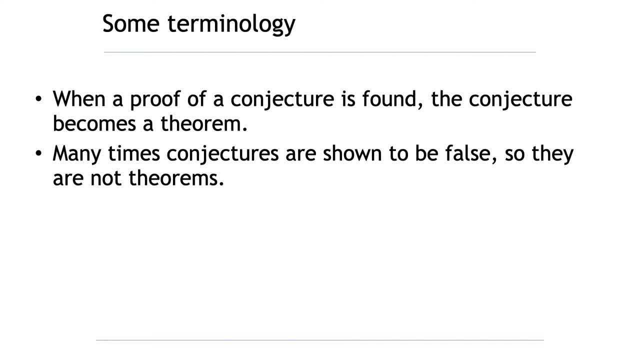 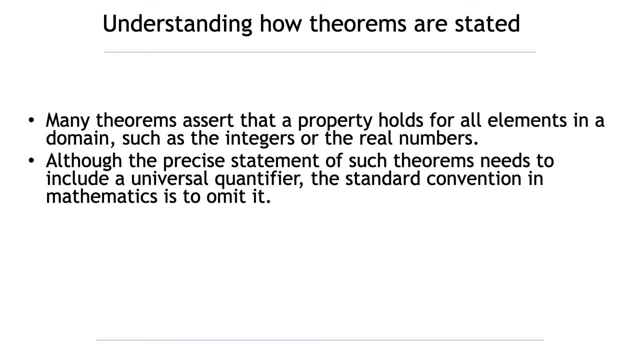 They are not like a proposition that can be either true or false. They are not like a proposition that can be either true or false. A theorem must always be true, otherwise it is not a theorem. Before we introduce methods for proving theorems: 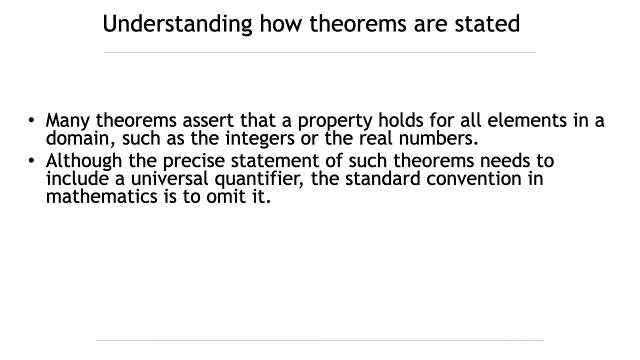 we need to understand how mathematical theorems are stated. Many theorems assert that a property holds for all elements in a domain, such as the integers or the real numbers, Although the precise statement of such theorems needs to include a universal quantifier. 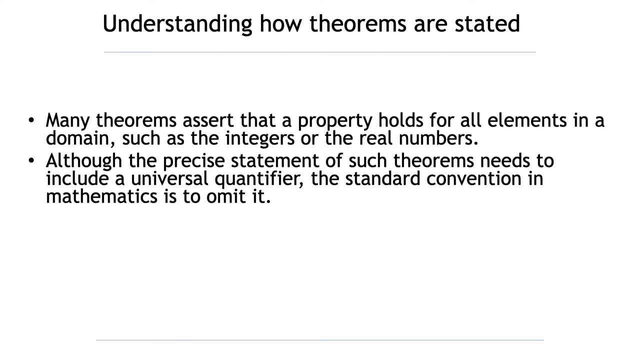 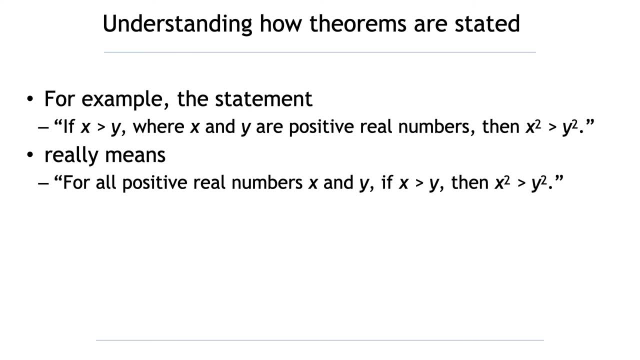 the standard convention in mathematics is to omit it. Then let's see an example, For example the statement: if x greater than y, where x and y are positive real numbers, then x squared is greater than y. squared really means for all positive real numbers, x and y. 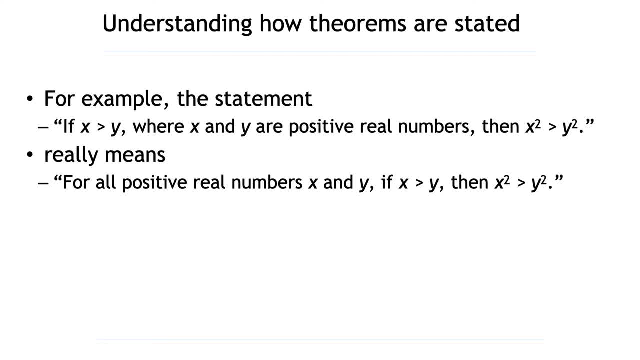 if x is greater than y, then x squared is greater than y squared. It is important to get this right. You will see these type of statements in many places and you need to understand the real meaning. Again, notice that in the statement. 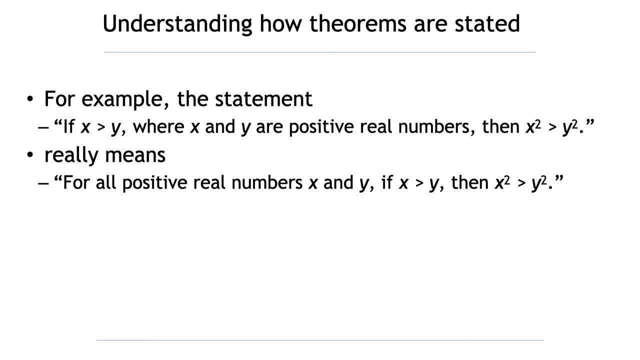 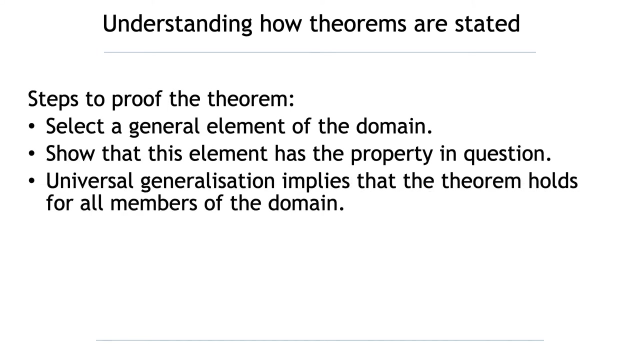 the first statement, we didn't use the universal quantifier. However, in that case the universal quantifier is implicit. We assume that the reader will know that the meaning of the statement is that it's valid for all positive real numbers To prove this type of theorem. 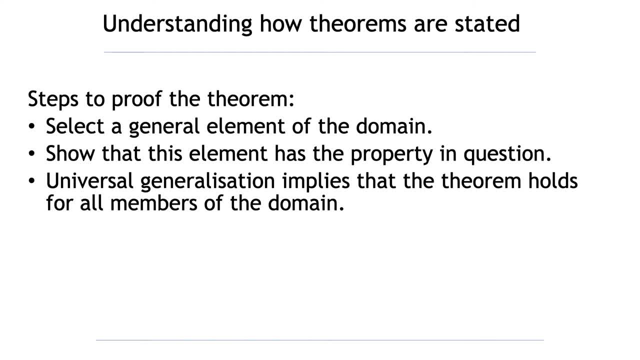 we usually follow three steps. We select the general element of the domain, Then we show that this element has a property in question. After that, universal generalization implies that the theorem holds for all members of the domain. These are the three common steps that we follow. 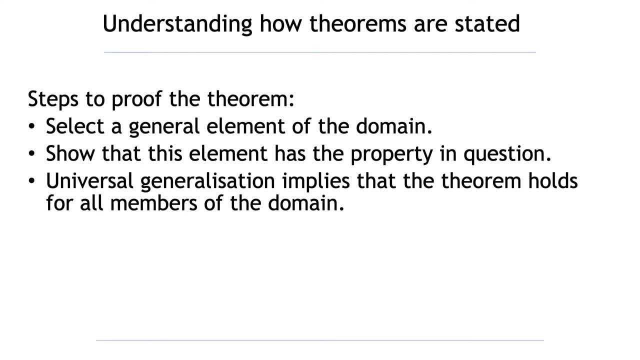 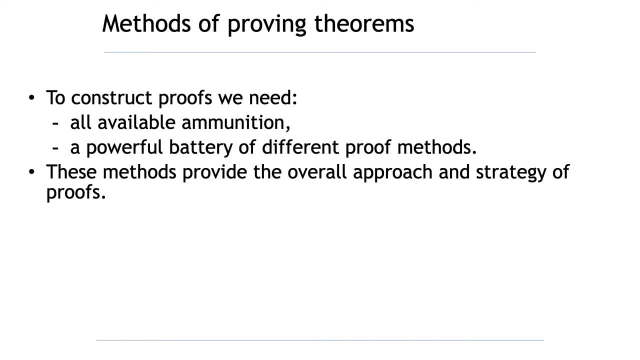 every time we want to prove the previous type of theorem, So proving mathematical theorems can be sometimes difficult. Therefore, we have to use all available ammunition that we can have, And we also need a powerful battery of different proof methods. These methods will provide the overall approach and strategy of proofs. 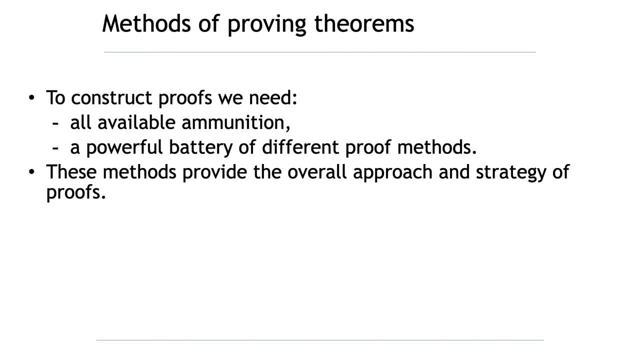 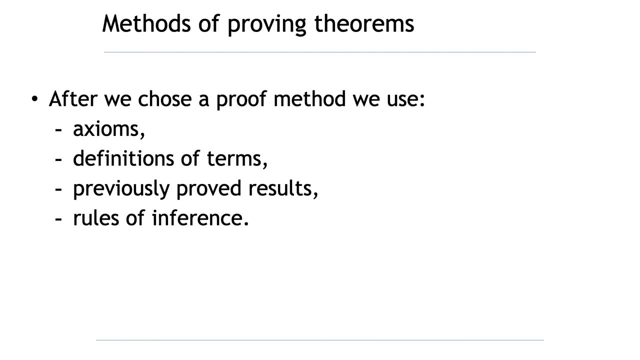 Understanding these methods is a key component of learning how to read and construct mathematical proofs. And, yes, you need to learn how to read proofs and also how to create them. When you construct your own proofs, be careful not to use anything but axioms, definitions. 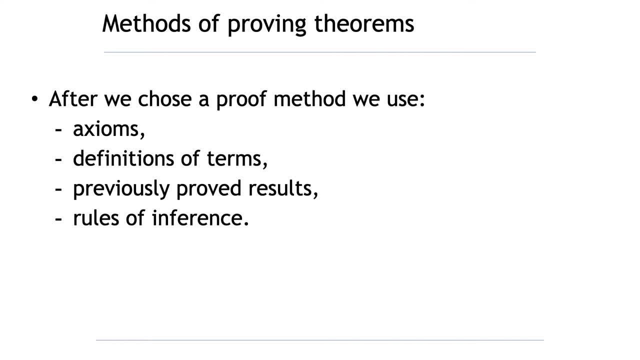 and previously proved results as facts. Remember everything you are going to use. it must be proved, Otherwise you will be making mistakes while proving your theorem. Therefore, what you believe is true is not true. Therefore, what you believe is true is not true. 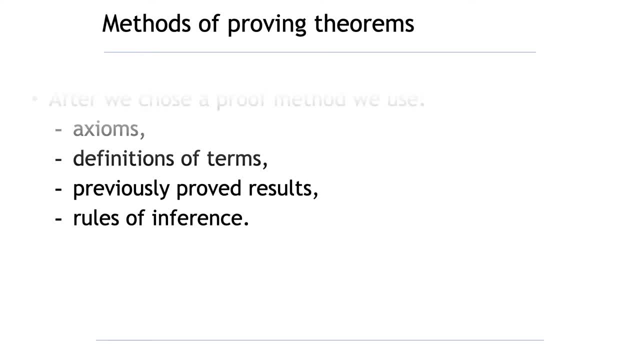 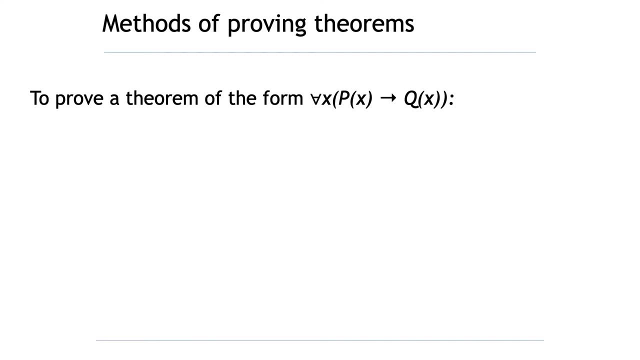 So in this case we need to show that the conditional statement is true. As you can see, the theorem has the form for rx: p at x implies q at x, So it is a conditional statement And we want to prove that this conditional statement is true. 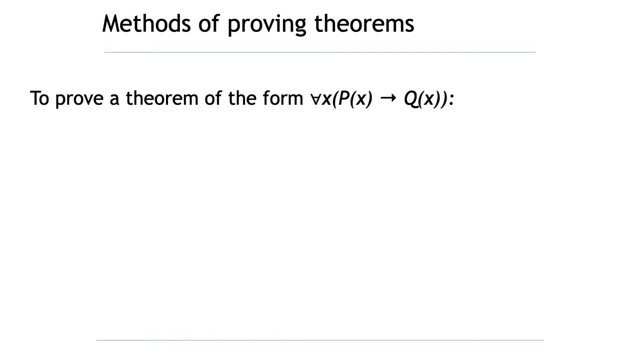 focus on methods that show that conditional statements are true. Our goal is to show that P at C implies Q at C is true where C is an arbitrary element of the domain. Remember, this is the first step: We choose an arbitrary element of the domain and we prove that the condition holds for that specific 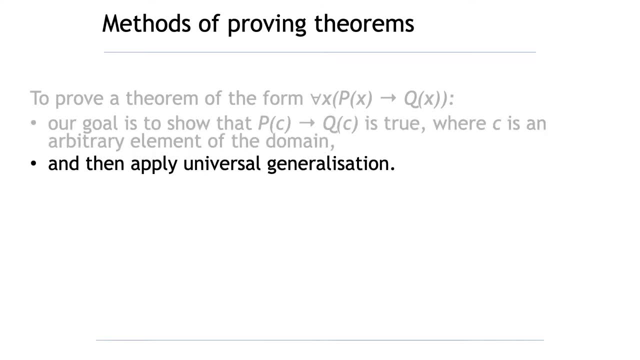 element. When we prove that, then we apply universal generalization. Recall that P implies Q is true. unless P is true but Q is false, Remember that We see that when we studied the truth. table for the conditional statement If you don't. 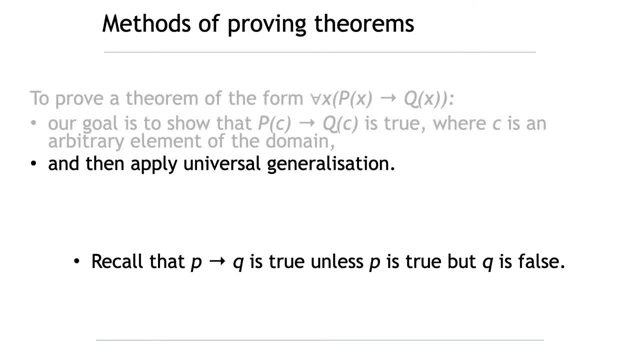 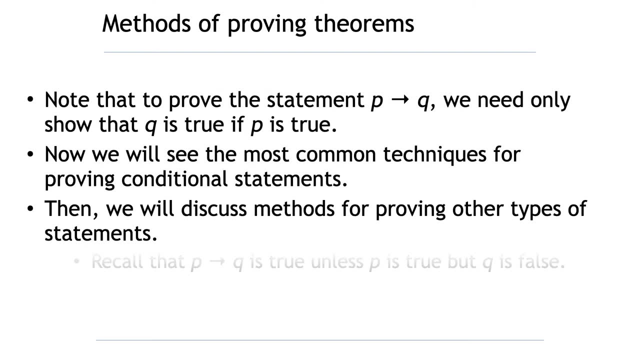 remember that you can go back to the video. of the video I'm going to leave the link below. in the description, Note that to prove the statement P implies Q, we need only to show that Q is true. if P is true. Now we will see the most common techniques for proving. 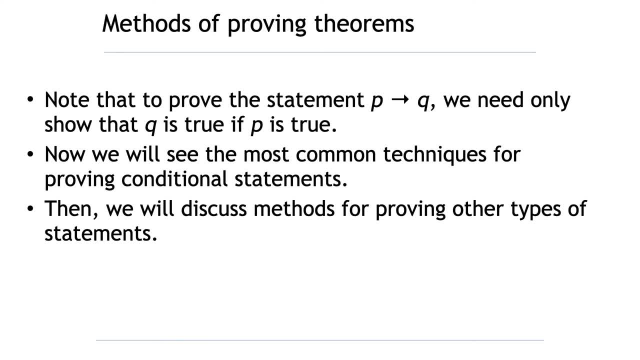 conditional statements. After that we will discuss methods for proving other types of statements. Remember, if you don't understand why to prove that P implies Q is true, we need only to show that Q is true. if P is true, please go back and see the truth table for the conditional. 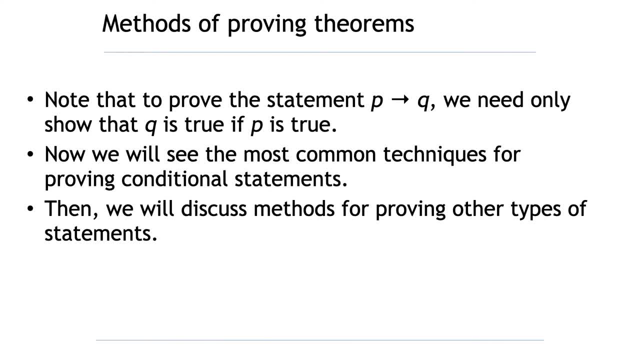 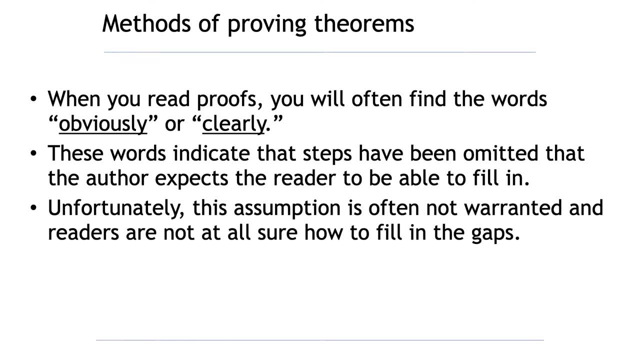 statement. Then you will realize that when Q is true, if P is true, is all we need to prove. When you read proofs, you will often find the words obviously or clearly. These words indicate that steps have been omitted that the author expects the reader to be able to fill in. Unfortunately, you must be very careful here. 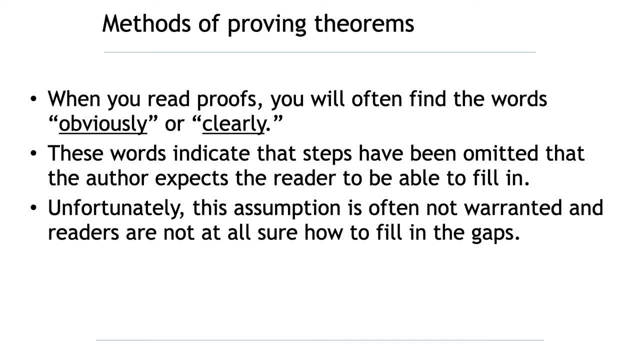 because this assumption is often not warranted and readers are not all sure how to fill in the gaps. Be especially careful if you are a student writing a test. In this case, you must make sure that the lecturer can fill in the gaps, so you will get good marks on. 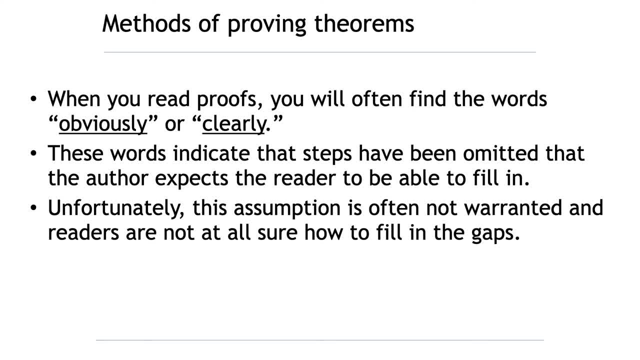 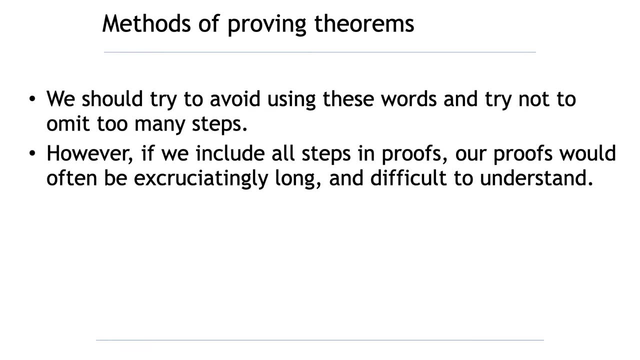 your solution. I always recommend the students not to skip any step, especially when they are being assessed, just to avoid unnecessary problems while the lecturer is marking the solutions. So we should try to avoid using these words and not to omit too many steps. We just want to avoid problems. However, if we include 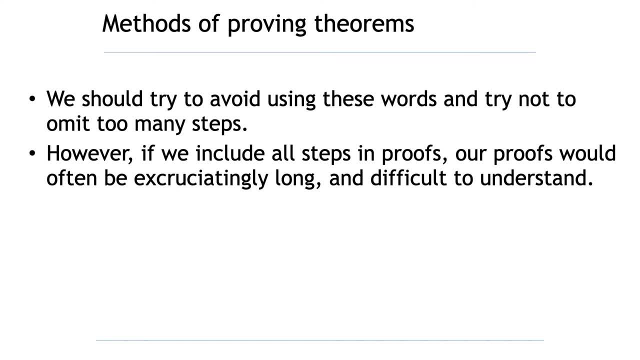 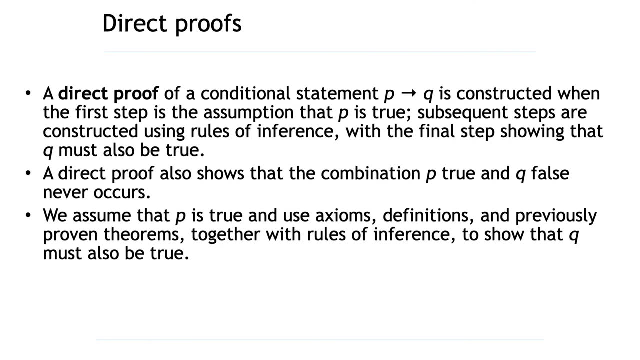 all the steps in certain proofs. our proofs will be often excruciatingly long and difficult to understand, So the key point here is to use the right balance in the right places. Let's see our first method to create a proof. A direct proof of a conditional statement- P implies Q- is constructed when the first step- 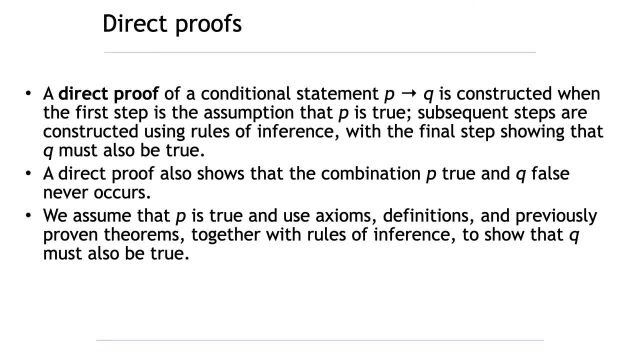 is the assumption that P is true. Subsequent steps are constructed using rules of inference, with the final step showing that Q must also be true. Remember that to create proofs, we usually have to make some assumptions. You already saw that type of proof. 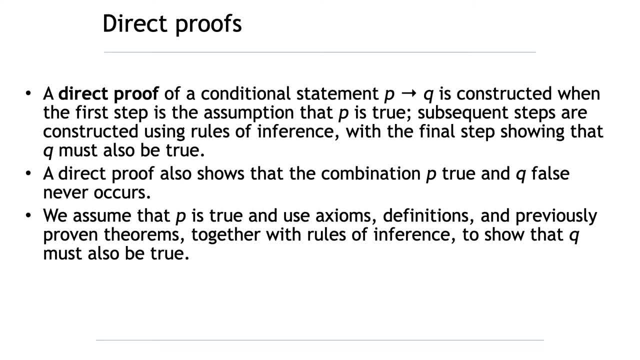 If you are not comfortable with rules of inference, I recommend you to watch the videos on the description that explain that specific topic. Do not go deeper in proofs without mastering rules of inference. A direct proof also shows that the combination P true and Q false never occurs. Why, As I 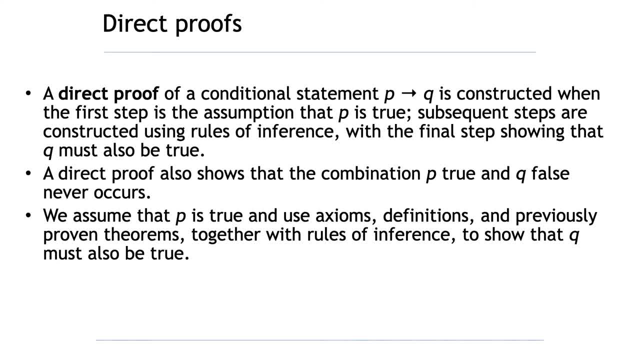 told you before. If you have any doubt on why these type of things can happen or are in that way, just please go and check the truth table for the conditional statement. You will see that P true and Q false give us as a result that P implies Q is false. 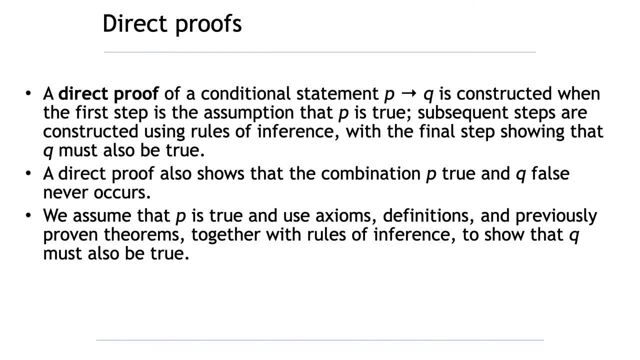 And because the theorem has to be always true, then that is what we have to show is that that combination never occurs. So we assume that P is true, and then we use axioms, definitions, previously proven theorems, rules of inference, and then we show that Q must also be true. If we do that, then we 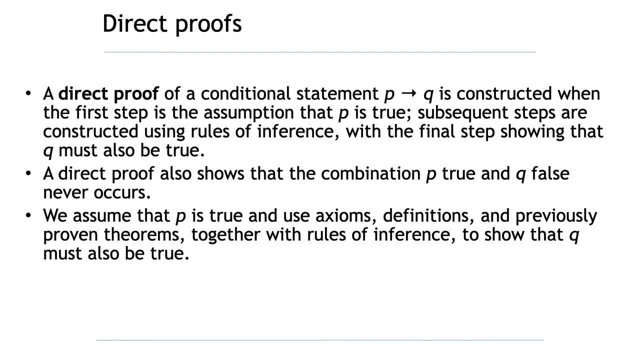 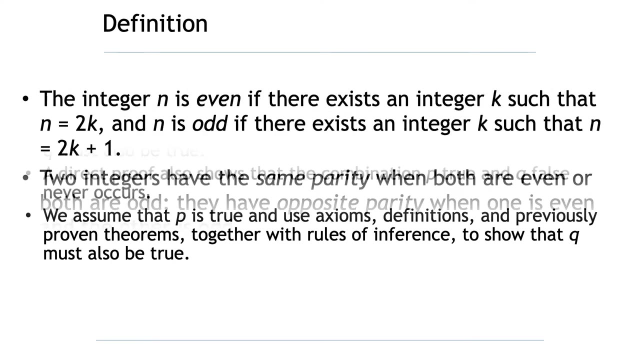 prove our theorem. Direct proofs of many results are quite straightforward, with a fairly obvious sequence of steps leading from the hypothesis to the conclusion. However, direct proofs sometimes require particular insights and can be quite tricky, as you will see in some of the examples. 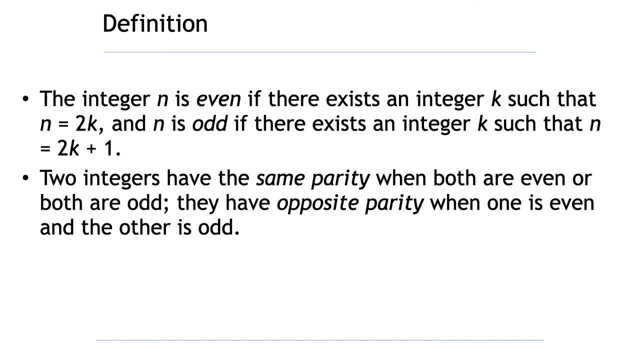 Let's see the following example: The integer n is, even if there exists an integer k such that n is equal to 2 times k and n is odd If there exists an integer k such that n is equal to 2 times k plus 1.. 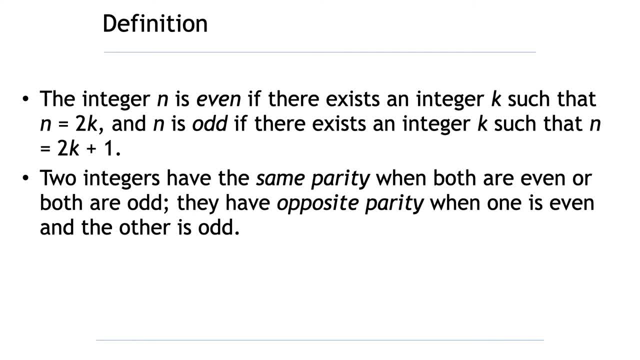 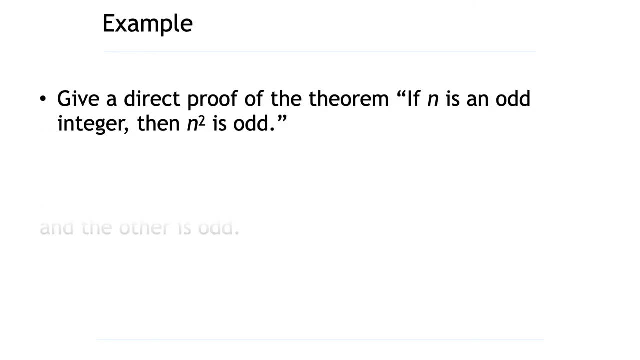 Two integers have the same parity when both are even or both are odd. They have opposite parity when one is even and the other is odd. This is our definition, and then we are going to state the theorem. So If we give a direct proof of the theorem, if n is an odd integer, then n squared is. 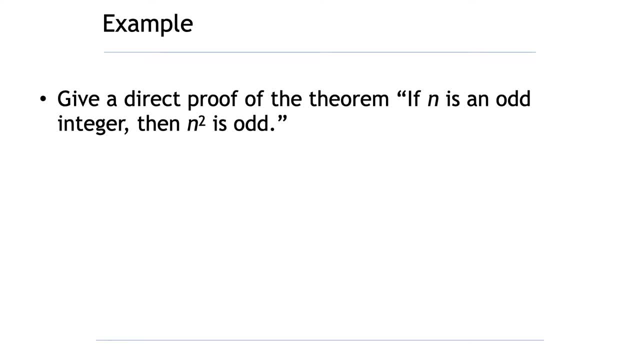 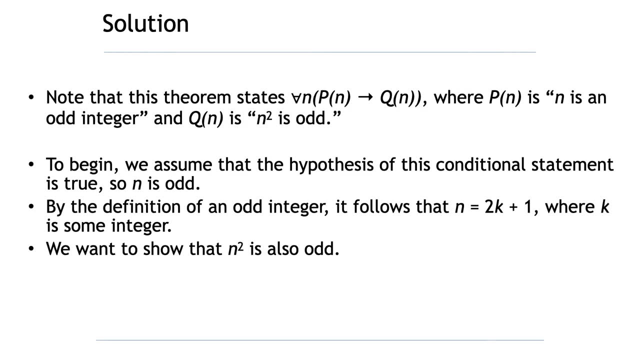 also odd. So now we have to prove that this theorem is true. Note that this theorem states that for all n, P and n implies Q at n. where P at n is n is an odd integer and Q at n is n squared. 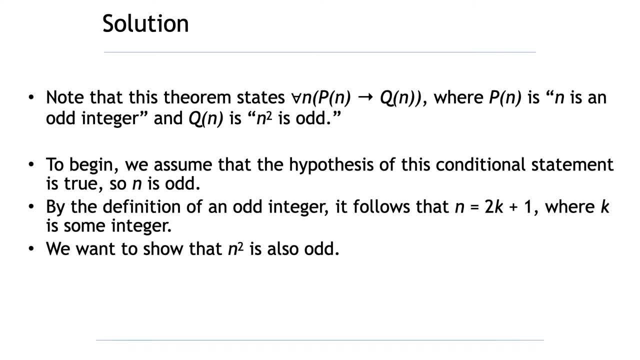 So we start here, assuming that the hypothesis of this conditional statement is true, which is P at n. So P at n is true. therefore n is odd. By the definition of an odd integer, it follows that n is equal to 2k plus 1, where k is some. 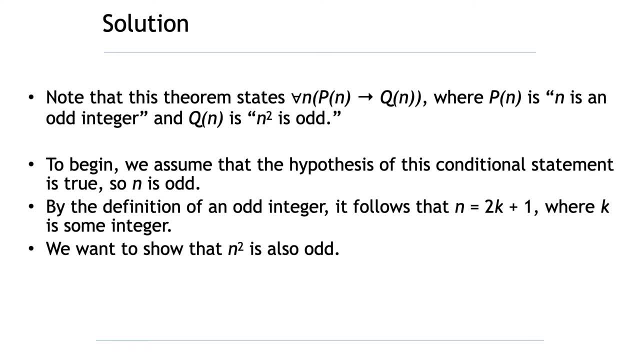 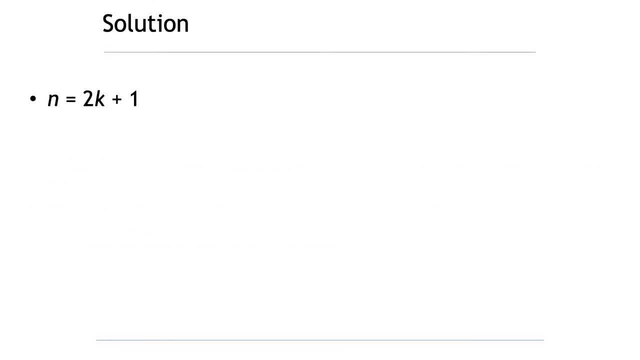 integer. We want to show that n squared is also odd. So we have our first equation: Because n is odd, then there exists a certain k, such that n equals to 2 times k plus 1.. If we square both sides of this equation, we get n squared equal to 2 times k plus 1. 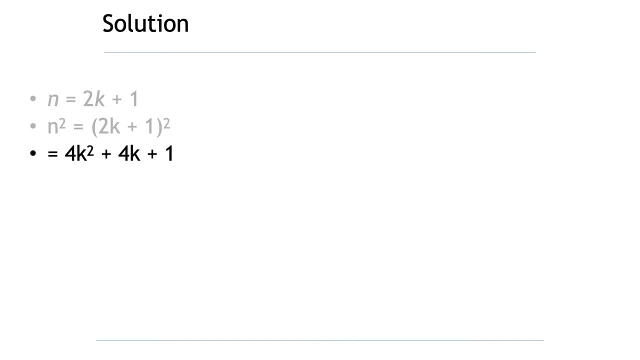 squared. OK, Now we can say that the result is the following: We can say that the result is the following: The right side of the equation is 4k squared plus 4k plus 1.. This is basic algebra. We just need to develop that right side of the equation. 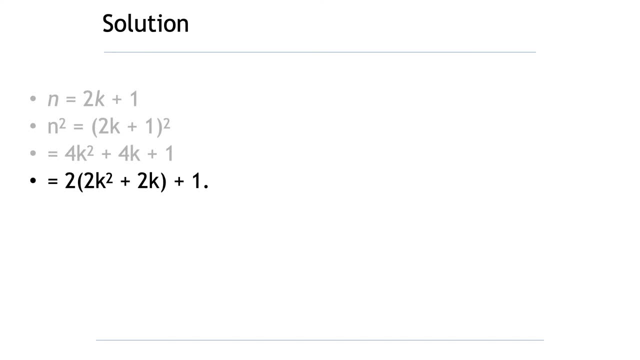 Now, if we choose a common factor between the first two terms as 2, this will give us a result that that 4k squared plus 4k plus 1 is also equal to 2 times 4k squared plus 1.. 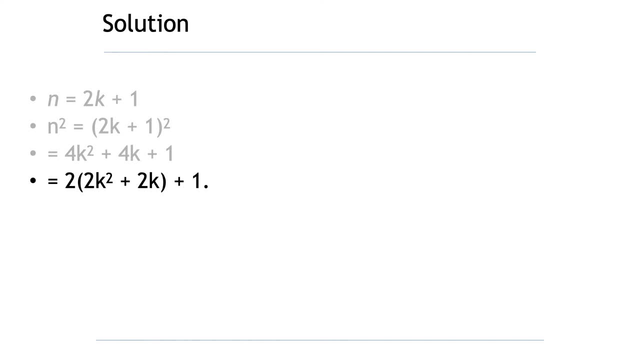 Now, by the definition of an odd integer, we can conclude that n? squared is also an odd integer. As you can see, n? squared is equal to 2 times a certain integer plus 1, which is the definition that we saw at the beginning of this exercise. 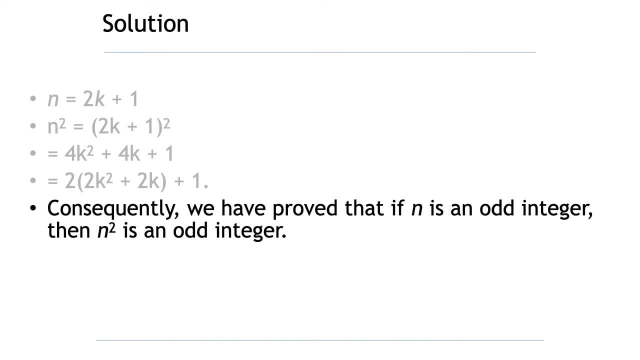 So, consequently, we have proved that if n is an odd integer, then n squared is also an odd integer. Notice that here we are doing a recap of a theorem as the last step. That's what you should always do. The last step of the proof must be a recap of the theorem. so you make your point very. 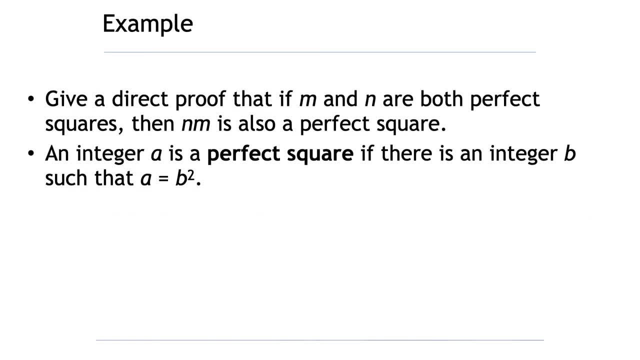 straight. Let's see another example. Give a direct proof that if m and n are both perfect squares, then n times m is also a perfect square. An integer a is a perfect square if there is an integer b, such that a equal to b squared. 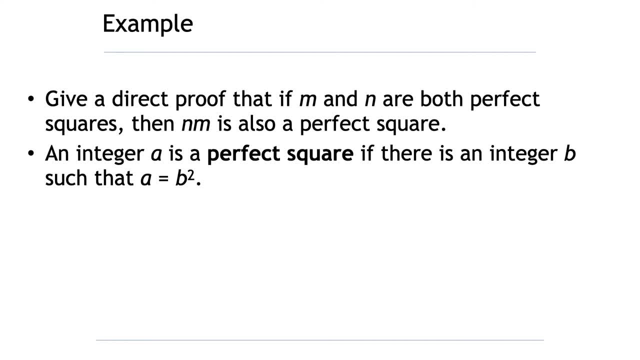 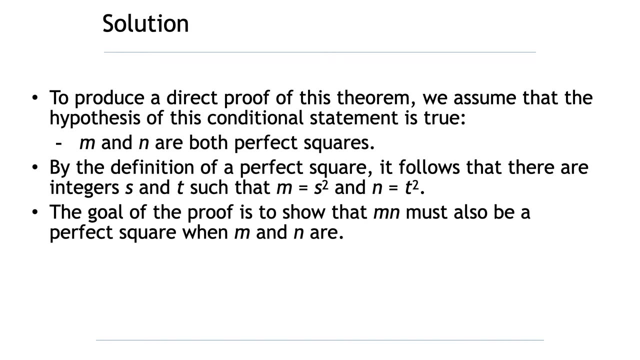 As you see in this example and from the previous one, we always have to state the definitions, so we know what exactly is what we have to prove. Again, to produce a direct proof of this theorem, we are going to use the three steps we mentioned. 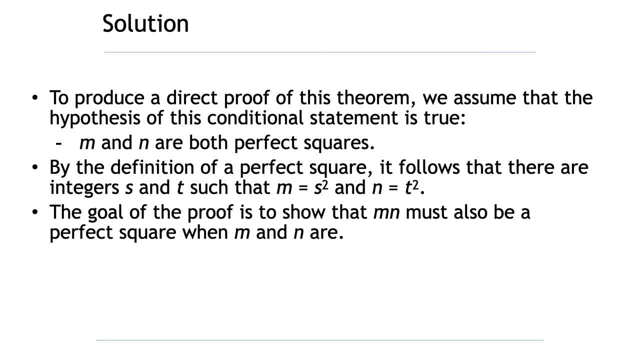 before. We are going to assume that the hypothesis is true, then m and n are both perfect squares. By definition of a perfect square, it follows that there are integers s and t, such that m is equal to s squared. So we know what exactly is what we have to prove. 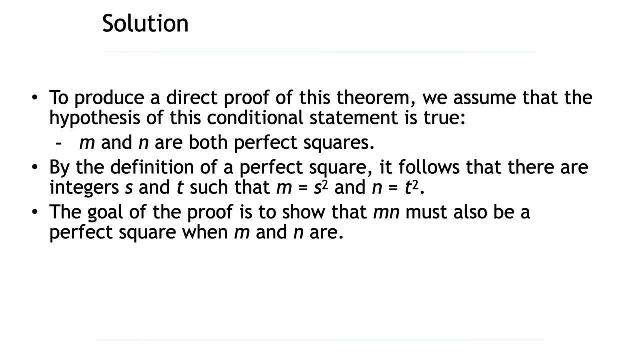 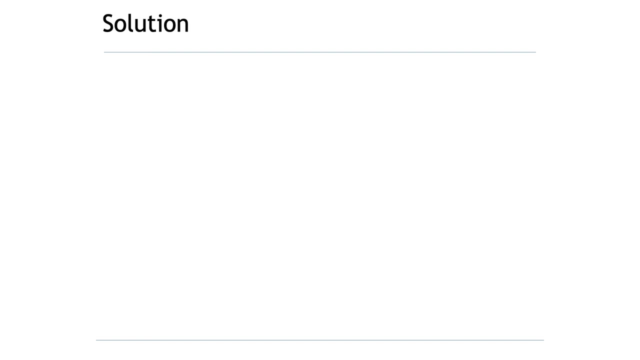 That's why it is important to have our definitions in place, because we usually have to use them to make the proof of a theorem. The goal of the proof is to show that m times n must also be a perfect square when m and n are. 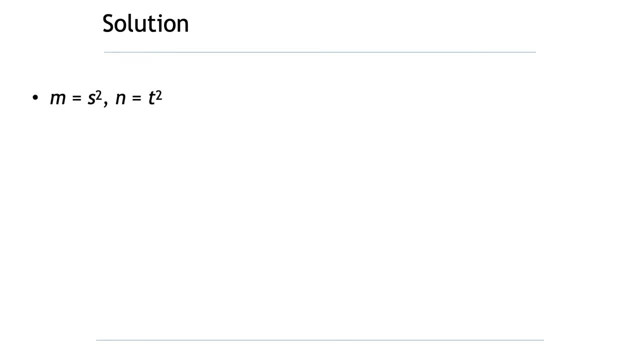 So let's see our solution: m is equal to s squared, n is equal to t squared. Remember, we are doing this because we are assuming that the hypothesis or the premise of the theorem is true. The third step is the following: S squared is equal to t squared. 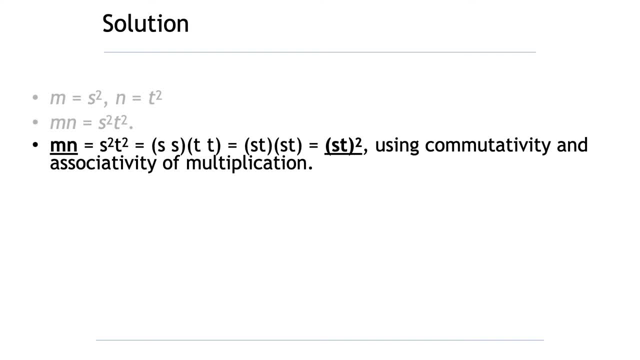 So we now develop the right side of that equation. We now have to work out what goes on at the right side of that equation. We now have to work out what goes on at the right side of that equation. So we will look at the right side of that equation. 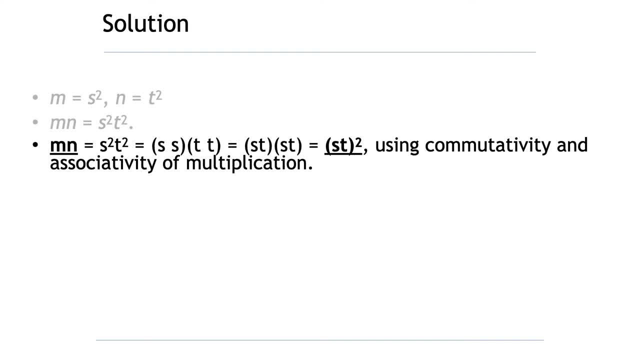 Let's previous example equation: s squared times t squared is the same or is equal to s times s times t times t. We can also say that s times s times t times t is equal to s times t times s times t. Here we are using the commutative and associativity of the 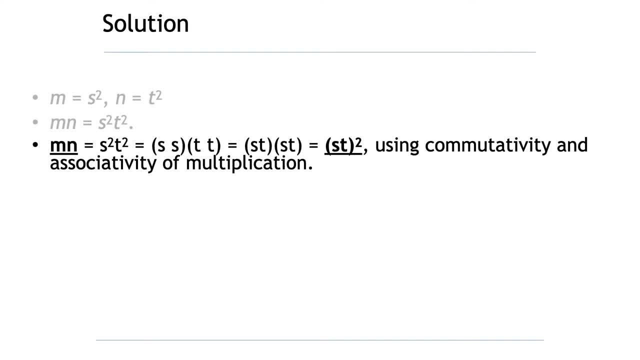 multiplication. Okay, remember, 2 times 3 times 4 is the same that 2 times 4 times 3.. Okay, those are rules that we don't need to explain, we don't need to prove them. Those can be used as axioms because those are results that are: 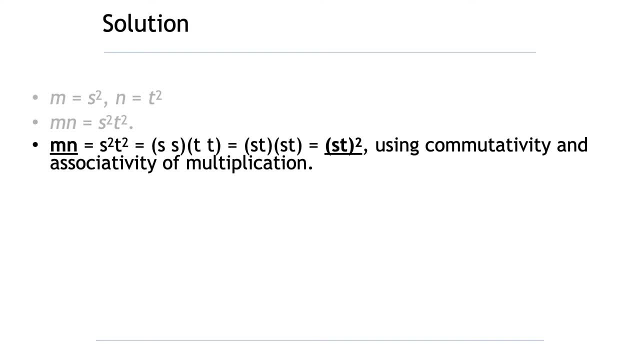 already been proved. So if we have now s times t times s times t, that is equal to s times t squared. Okay, then we have that n times n is equal to the square of a certain number. So by definition of a perfect square, it follows that 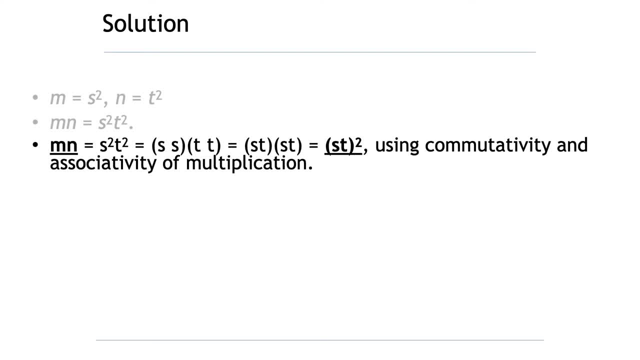 n times n is equal to the square of a certain number. So by definition of a m times n is also a perfect square. okay, because it is the square of s times t, which is an integer. we have proof that if m and n are both perfect squares, then m times n is also a perfect square. 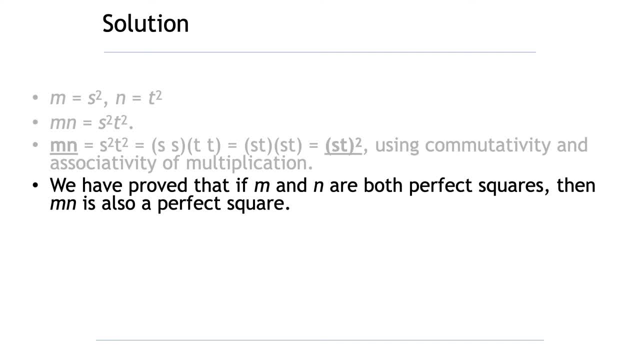 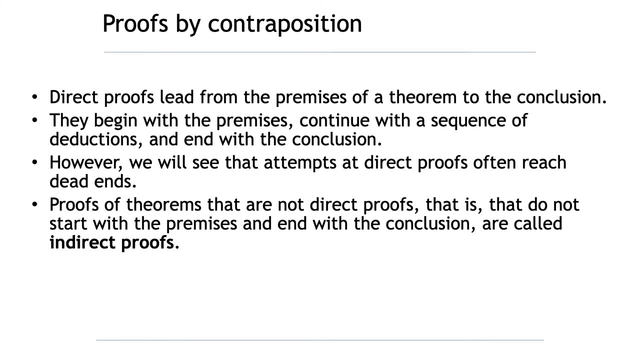 as you can see, here again we are doing a recap of the theorem, just to make sure that our point is very straight. as we saw in the previous examples, direct proofs lead from the premises of a theorem to the conclusion. they begin with the premises, continue with the sequence of deductions. 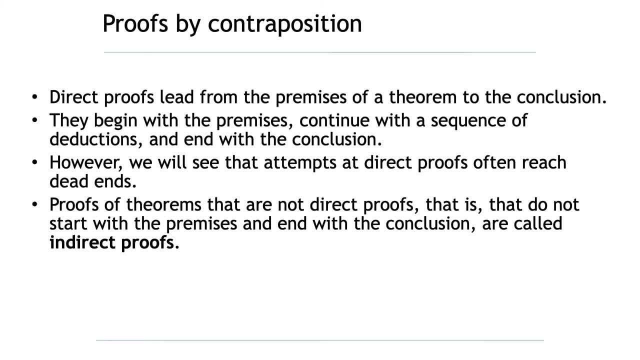 or logical steps and end with the conclusion. however, we will see that attempts at direct proofs often reach dead ends. so what can we do in that case? so in that case we are. we have to use another strategy. proof of theorems that are not direct proofs, that is, that do not start with the premises and end with the conclusion, are called indirect. 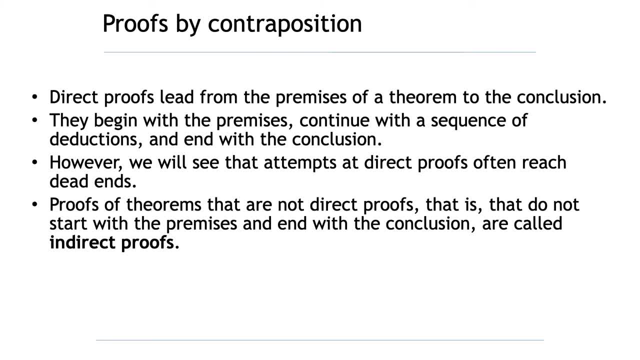 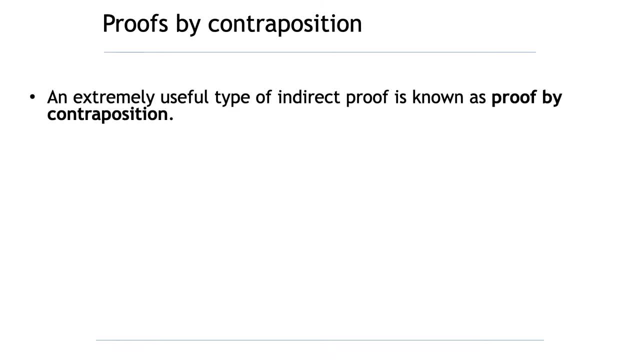 proofs. we are going to see now examples of this type of proof. an extremely useful type of indirect proof is known as proof by contraposition. so remember that when we studied logical equivalences, we saw that the contrapositive of the conditional statement is logically equivalent to the conditional statement in another way. the conditional 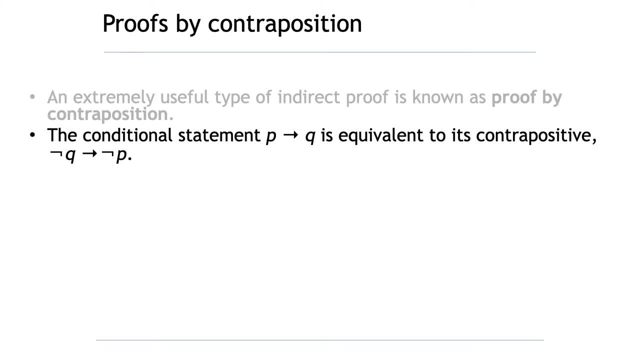 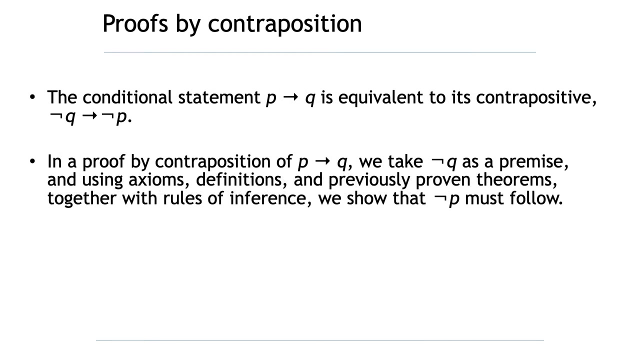 statement p implies q is logically equivalent to its contrapositive no q implies no p. therefore, the conditional statement p implies q can be proved by showing that its contrapositive no q implies no p is true. In a proof by contraposition of P implies Q, we take node Q as a premise and then we 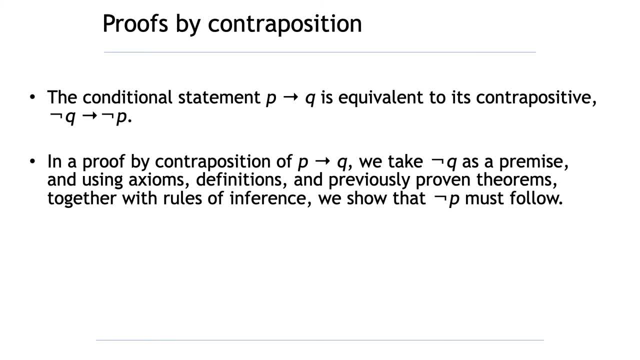 use axioms, definitions and previously proven theorems, together with rules of inference, and we show that node P must follow In another way. we first transform our theorem using the contrapositive and then we just make a direct proof. Let's see the following example: 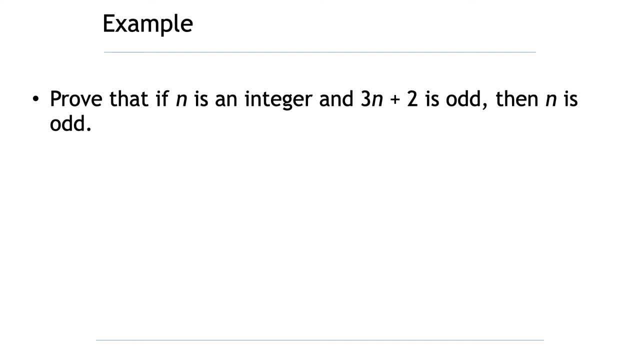 Proof that if n is an integer and 3 times n plus 2 is odd, then n is also odd. We first attempt a direct proof. We assume that 3n plus 2 is an odd integer. This means that 3n plus 2 is equal to 2k plus 1 for some integer. 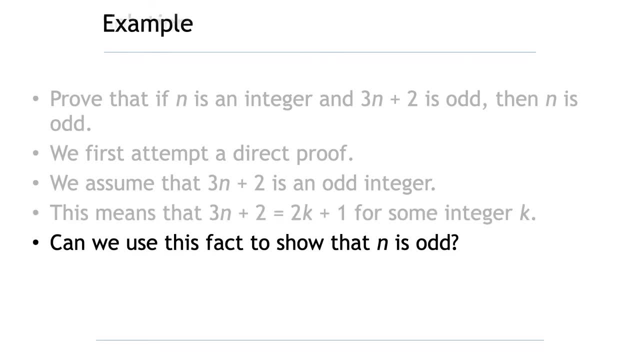 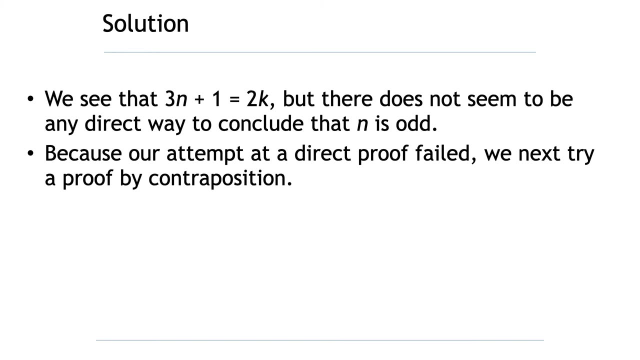 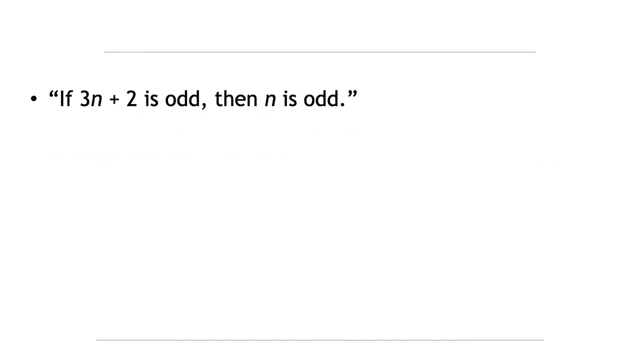 Now we can see that 3n times 1 is equal to 2k, but there doesn't seem to be any direct way to conclude that n is odd Because our attempt at a direct proof failed. we next try a proof by contraposition. 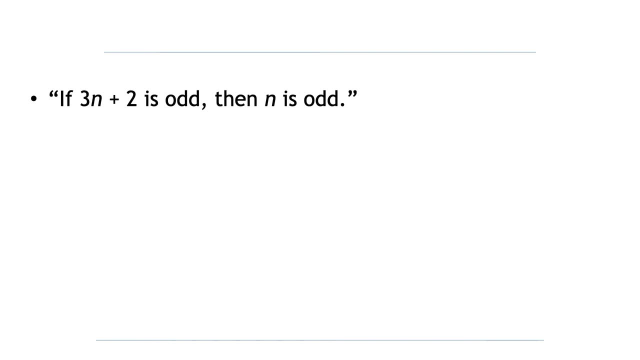 So this is our theorem: If 3n plus 2 is an integer, then 3n plus 2 is an odd integer. If 3n plus 2 is an integer, then 3n plus 2 is an odd integer. 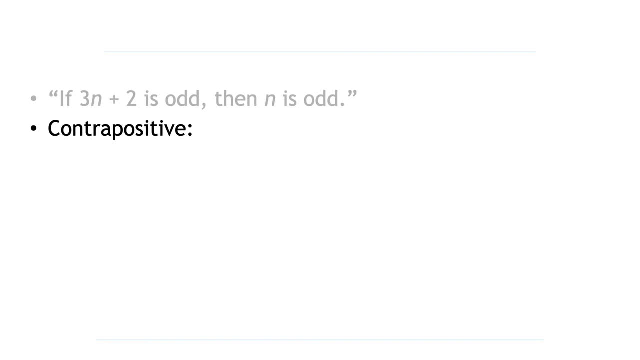 If 3n plus 2 is odd, then n is odd. Now the contrapositive will be: if not n is odd, then not 3n plus 2 is odd. We can write this in a better way: We just say that n is even, then 3n plus 2 is also even. 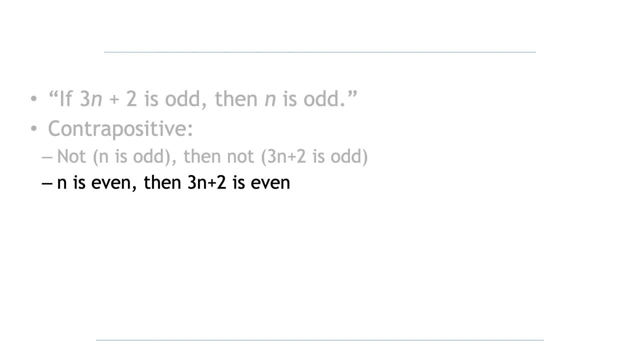 This is the contrapositive of your theorem. Now let's try to prove the contrapositive By definition of an even integer n is equal to 2k for some integer k. So if we substitute 2k for n, we are going to get this equation. 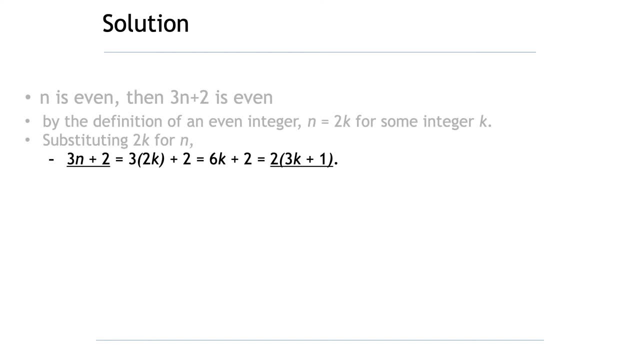 If you see 3n plus 2, we substitute n by 2k. we get 3 times 2k plus 2.. That is also equal to 6k plus 2.. And if we extract 2 as the common factor between the two terms, we are going to get 2 times. 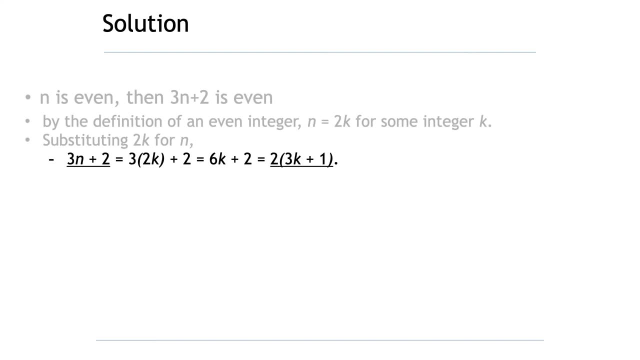 3k plus 1.. So now This tells us that 3n plus 2 is even- because it's 2 times some- integer, and therefore it's not odd. This is the negation of the premise of the theorem. 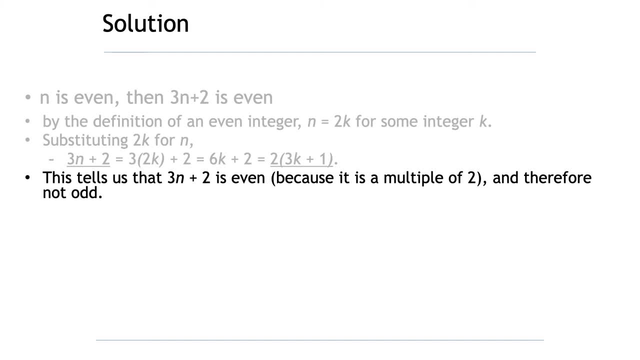 Because the negation of the conclusion of the conditional statement implies the hypothesis is false in other way, not Q implies not P, then the original conditional statement P implies Q is true. We just proved that the theorem if 3n plus 2 is odd, then n is odd. 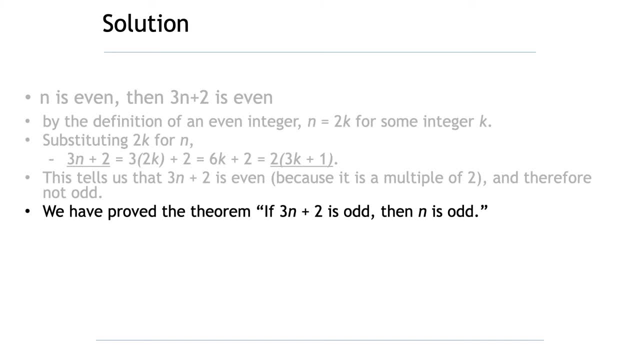 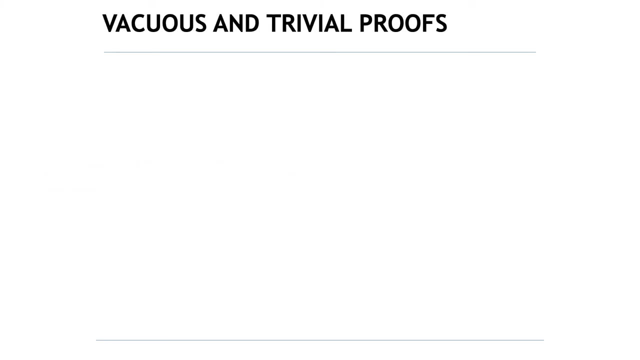 As you see, here again we are doing a recap of the theorem to state that we finished the proof. So there is another type of proof that is called vacuous and trivial proofs. So For we to understand this type of proof, let's use the truth table of the conditional. 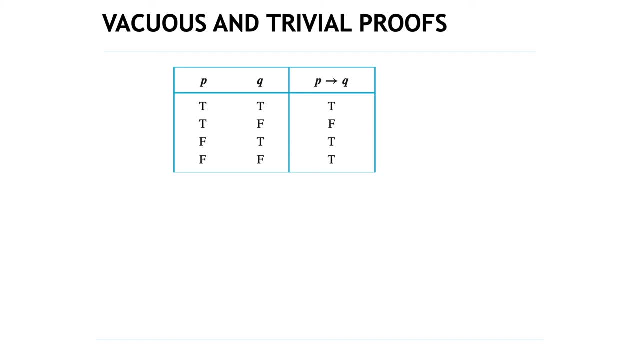 statement, the one that I mentioned before in several times. As you can see, every time that P is false, then P implies Q is true. Can you see that? So we have two rows that p is true and we have two rows that p is false in the two rows that. 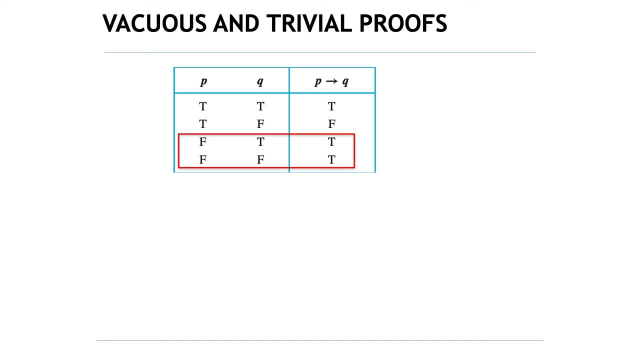 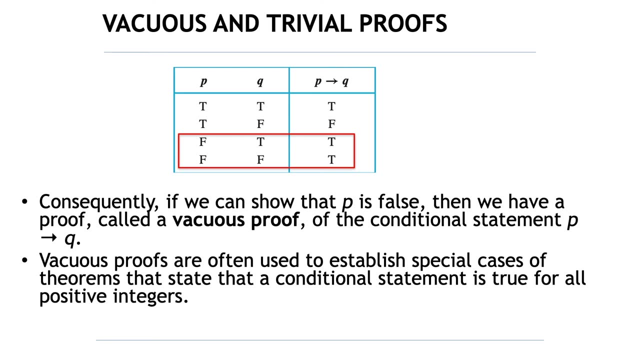 p is false. it doesn't matter what the value of q is. the conditional is always true. consequently, if we can show that p is false, then we have a proof. okay, we just prove that the conditional will be true. this type of proof is called the vacuous proof on the conditional statement. 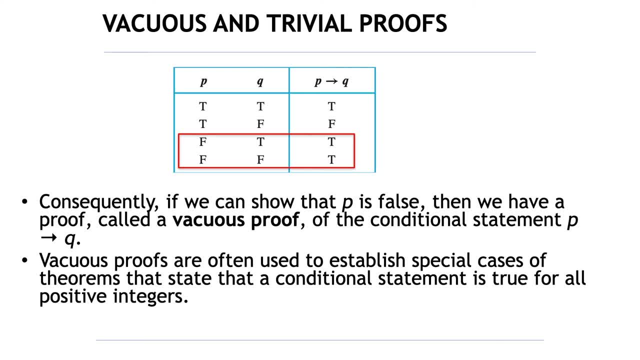 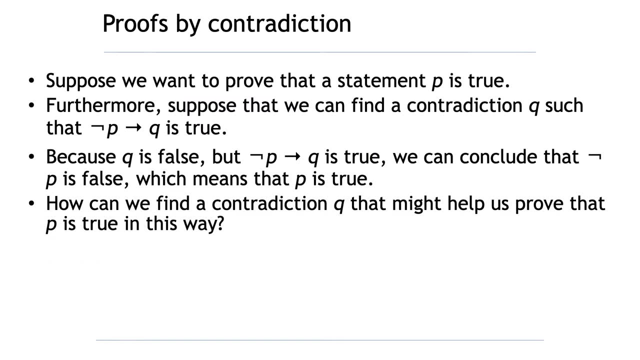 p implies q. so this type of proof is often used to establish special cases of theorems that state that the conditional statement is true for all positive integers, for instance. we also have another type of proof that is called proof by contradiction. suppose we want to prove that the statement p is true. furthermore, suppose that we can. 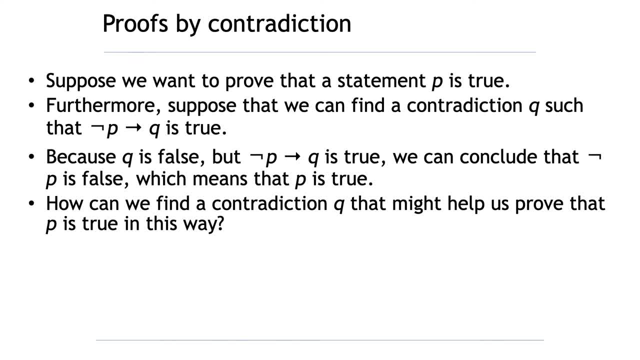 find a contradiction q such that no p implies q is true, because q is false, but no p implies q is true, we can conclude that no p is false, which means that p is true. how can we find a contradiction q that might help us to prove that? 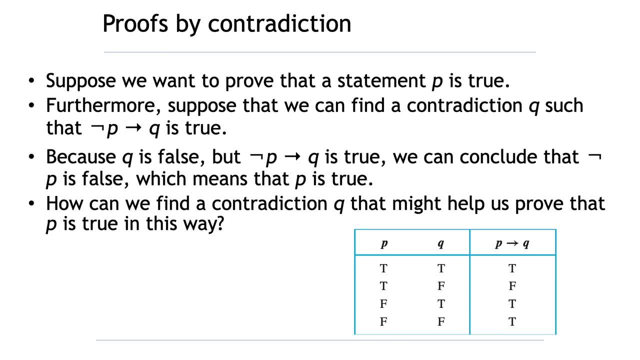 p is true. in this way it is actually quite easy- and it's one of the tricks that sometimes we want, we have to use to make certain proofs again. as you can see in the truth table for the conditional statement to be true: when q is false, then p has to be false. if we prove that no p implies q is true, then 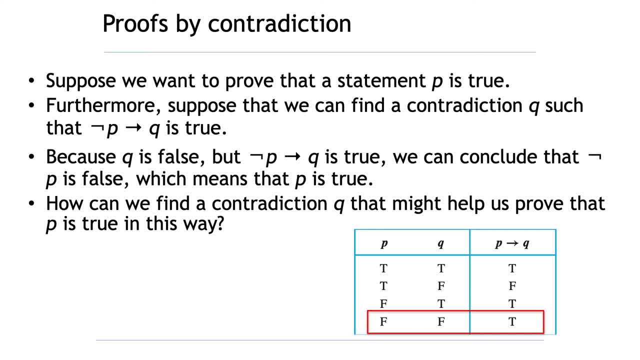 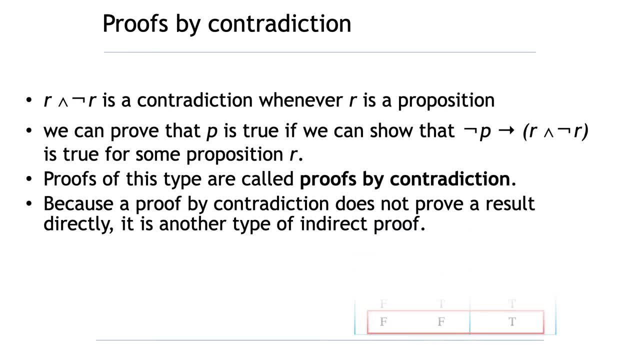 false, then no P has to be false. If no P is false, then P is true. and we just prove our theorem. We already know that R and no R is a contradiction whenever R is a proposition. We studied that before in the previous videos. Now we can prove. 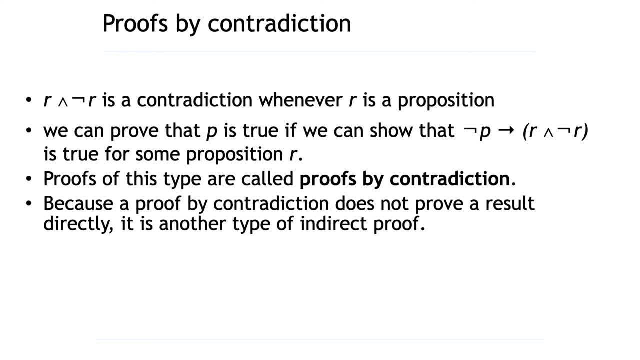 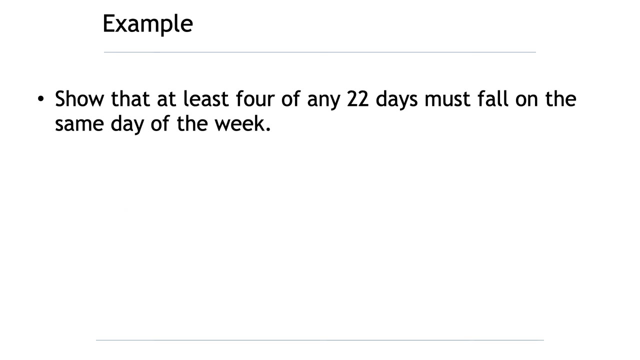 that P is true if we can show that no P implies R and no R is true for some proposition R. Proof of this type are called proofs by contradiction. because the proof by contradiction does not prove the result directly, it is another type of indirect proof. Let's see the following example: Show that at least. 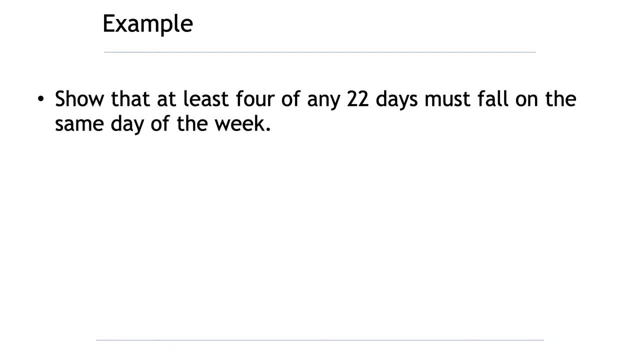 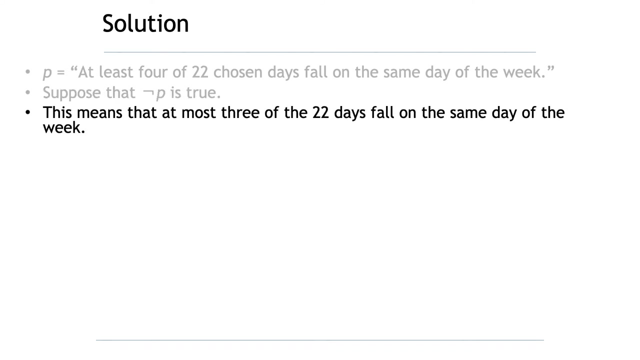 four of any 22 days must fall on the same day of the week. Let P be the proposition. at the least four of 22 chosen days fall on the same day of the week, If we choose. you're supposed to prove now that no p is true. This means that at most three of the 22 days fall on the same way of the. 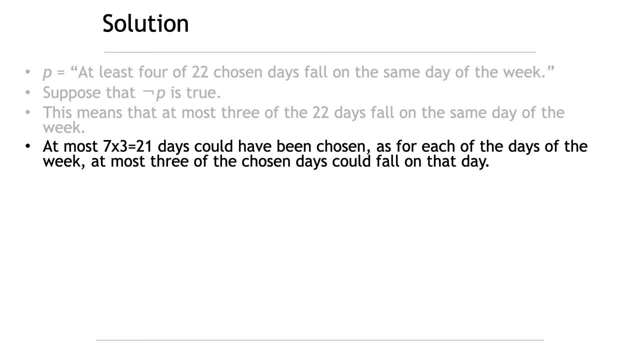 week, If we choose at most three days and a week have seven days, at most 21 days could have been chosen. At most three of the chosen days could fall on that day. This contradicts the premise that we have 22 days under consideration. We just saw before that now we only can have at maximum. 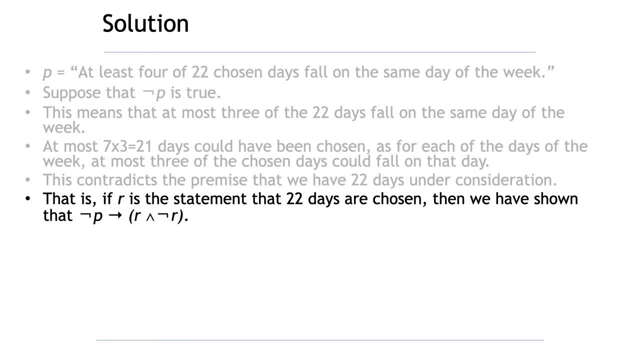 21 days. That is, if r is the statement that 22 days are chosen, then we have shown that no p implies r and no r, which is a contradiction. Consequently, we know that p is true. We just proved that at least. 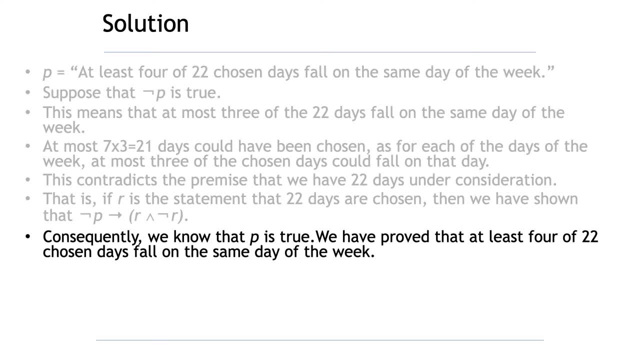 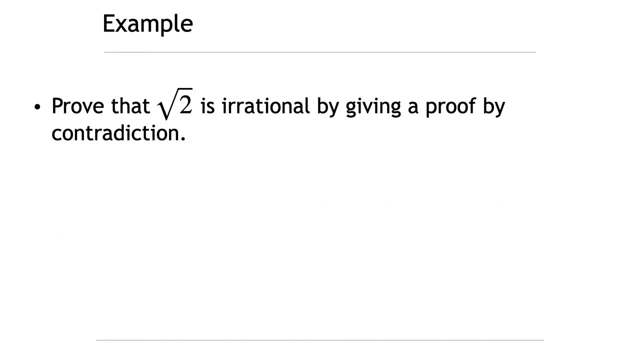 four of 22 chosen days fall on the same day of the week. Again, as you can see, the last step of the proof is to recap the theorem. Never forget to do that. Let's see another example. Prove that square root of 2 is irrational by giving a proof by: 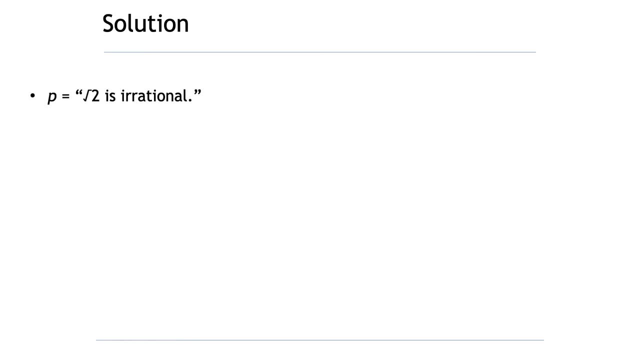 contradiction. So let's p be the proposition. square root of 2 is irrational. To start a proof by contradiction, we suppose that no p is true. If r is the statement that 22 days fall on the same day of the week, then no p is true. Then no p is. it is not the case that square root of 2 is irrational. 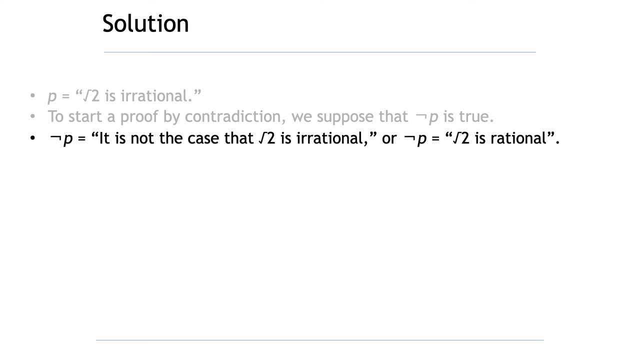 or no p is equal to square root of 2 is rational. Let's now show that assuming that no p is true leads to a contradiction. If square root of 2 is rational, there exist integers a and b with square root of 2 equal to a divided by b, where b is different than 0, and a and b have no common. 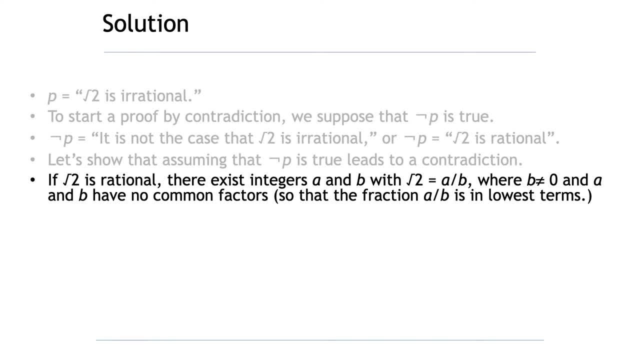 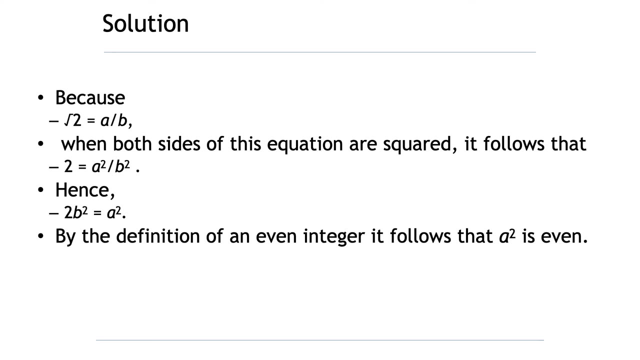 factors. So that means that the fraction a divided by b is in its lowest terms. You cannot make it a and b any smaller number, Because square root of 2 is equal to a divided by b. when both sides of this equation are square root of 2, equal to a divided by b, then the fraction a divided by b is: 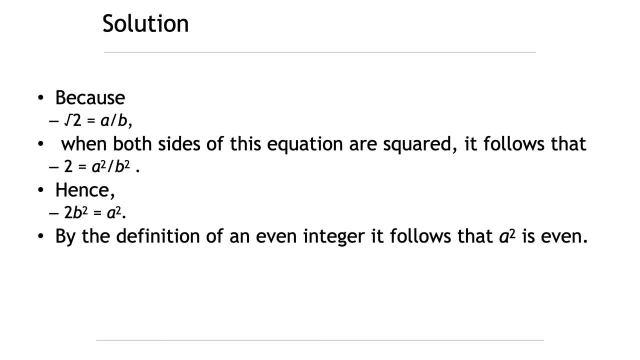 equal to a squared. It follows that 2 is equal to a squared divided by b squared. Hence 2b squared is equal to a squared. Here we are just transforming the equation, We didn't do anything else. By definition of an even integer, it follows that a squared is even. We proved that before. So next: 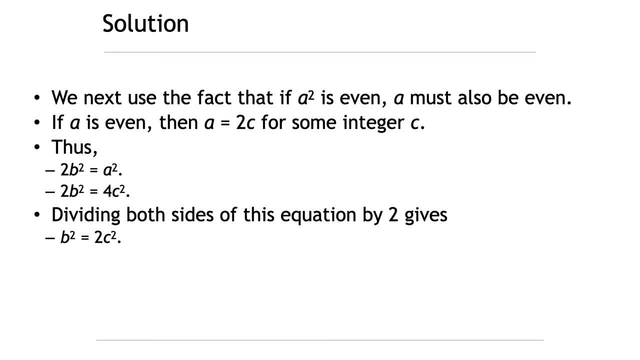 we use that the fact that a squared is even a must also be even If a is even, then a is equal to 2c for some integer c. Thus 2b squared equal to a squared. we can transform that in: 2b squared equal to. 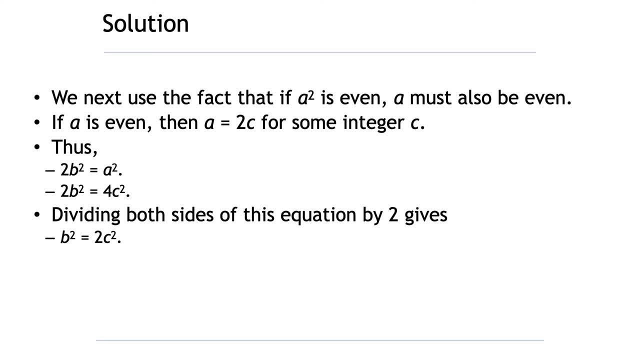 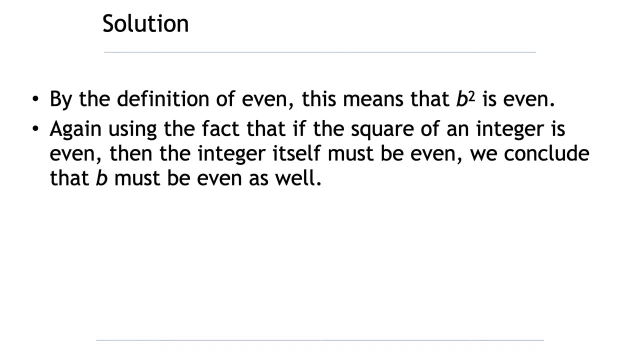 4c squared. Dividing both sides of this equation by 2, it gives us, as a result, that b is equal to a squared. that b squared is equal to 2 times c squared. By definition of even, this means that b squared is even. 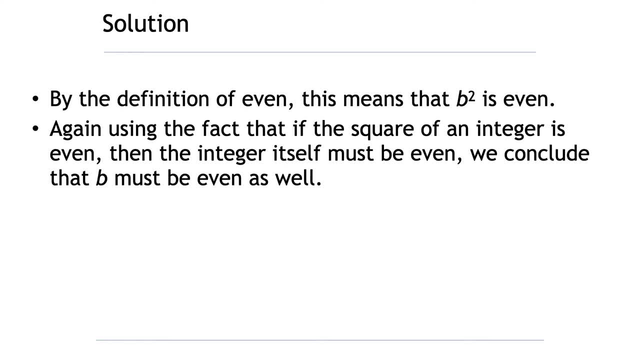 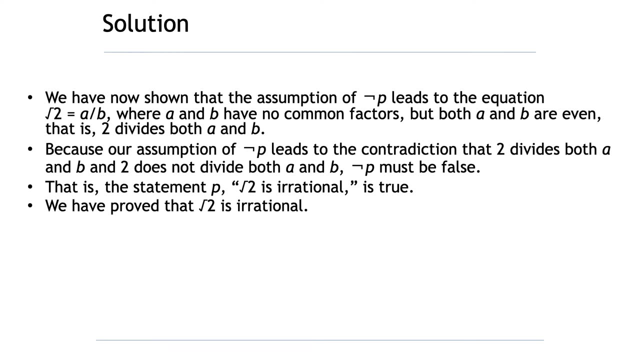 Again, using the fact that if the squared of an integer is even, then the integer itself must be even, We conclude that b must be even as well. So what? we have now shown that the assumption of no-p leads to the equation square root of 2 equal to a divided by b, where a and b have no common. 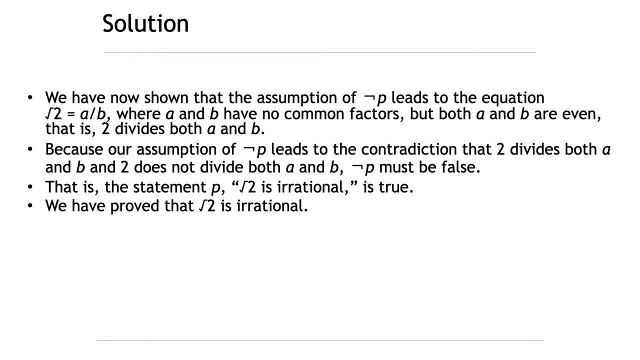 factors, but both a and b are even. that is, 2 divides both a and b. So the statement square root of 2 equals to a divided by b, where a and b have no common factors, is even. instead it is just two. That is, 2 divided by a. divided by b equals to 1. preparation not related together. 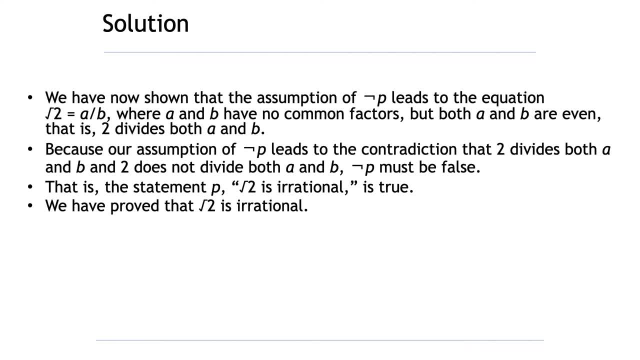 Please fuck all none and please leave your comments. Thanks for watching. If this result was useful for you, comment below, Like and share this video for others. Thank you bye. common factors means that, in particular, 2 does not divide both a and b. 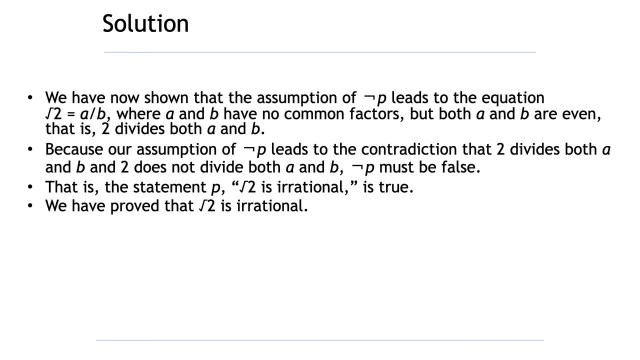 Because our assumption of no p leads to the contradiction that 2 divides both a and b and 2 does not divide both a and b. no p must be false. That is, the statement p, square root of 2 is irrational is true. We have proof, therefore, that square root of 2 is irrational. 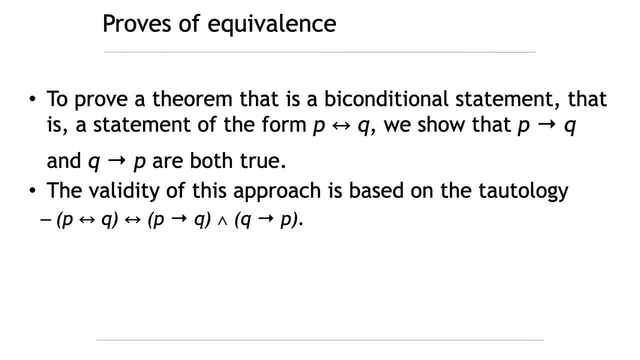 To prove a theorem that is a bi-conditional statement, that is a statement of the form p if and only if q. we show that p implies q and q implies p are both true. The validity of this approach is based on the tautology: p if and only if q. 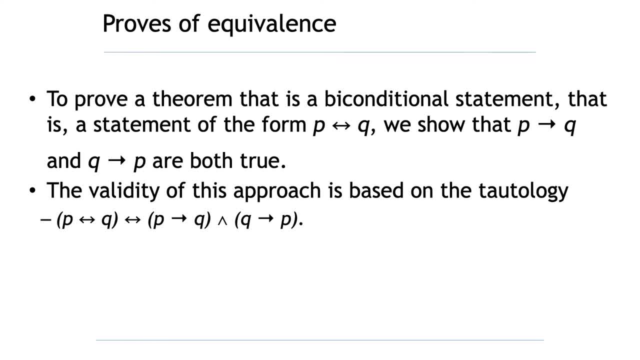 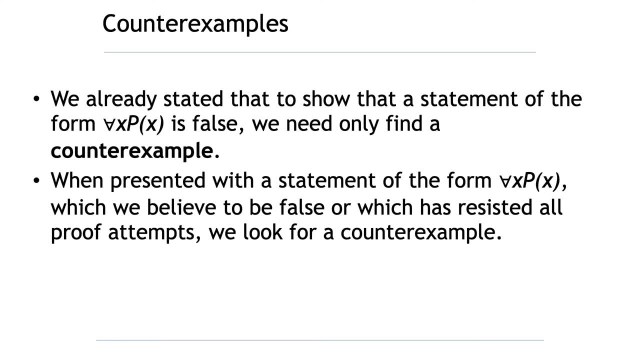 if, and only if, p implies q and q implies p. We already stated before that, to show that statement of the form for all x, p at x, is false, we need only to find a counterexample When presented with statements of the form for all x, p at x, which we believe to be false or which has. 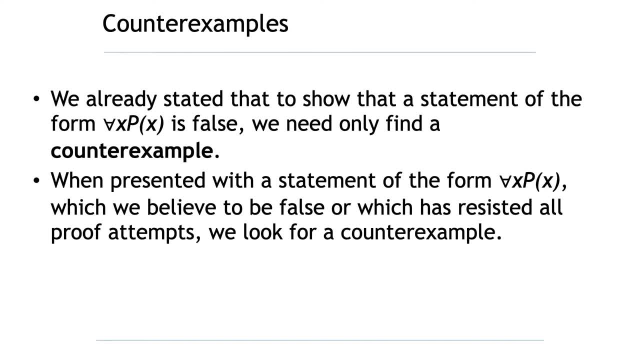 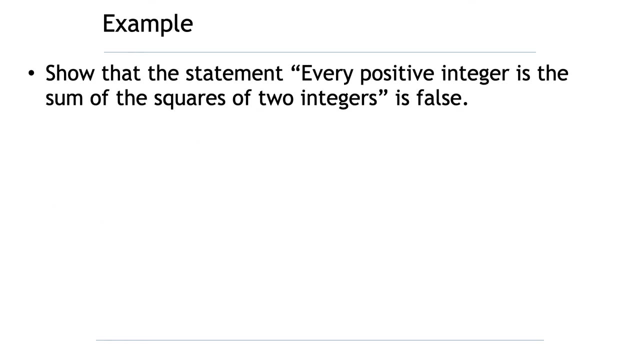 resisted all proof attempts, then we look for a counterexample. Many times in mathematics, counterexamples are used to prove that certain statement is false. So this will be another technique that we will have in our arsenal when we are working with proofs. Let's see an example. Show that the statement every 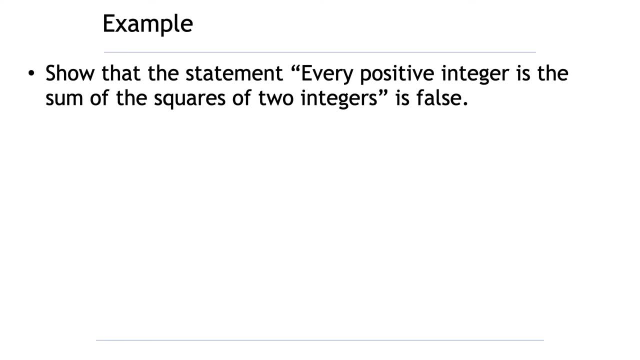 positive integer is the sum of the square of two integers is false. We look for a particular integer that is not the sum of the squares of two integers. 3 cannot be written as the sum of the square of two integers, To show that know. 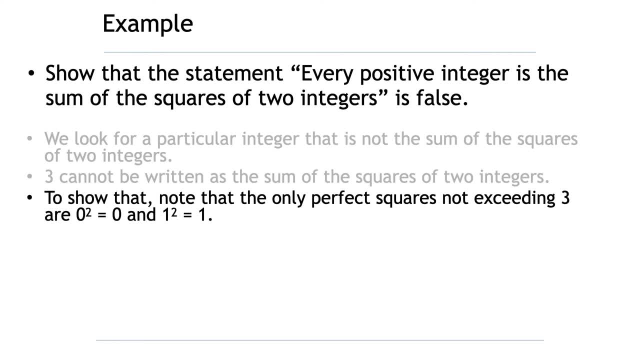 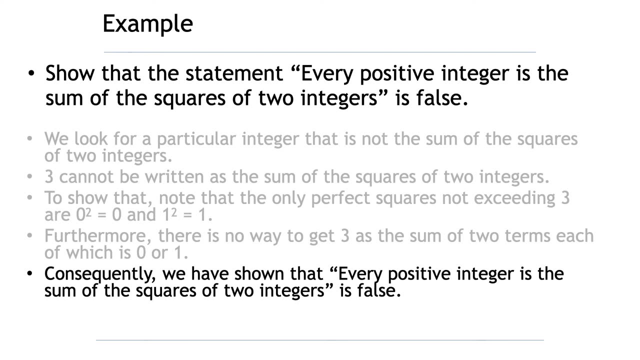 that only perfect squares not exceeding 3 are 0 or 0.. and one. Furthermore, there is no way that to get three as the sum of the two terms, each of which is zero or one. Consequently, we have shown that every positive integer is the sum of the. 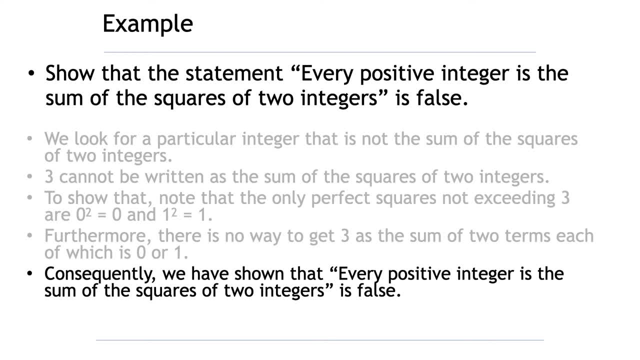 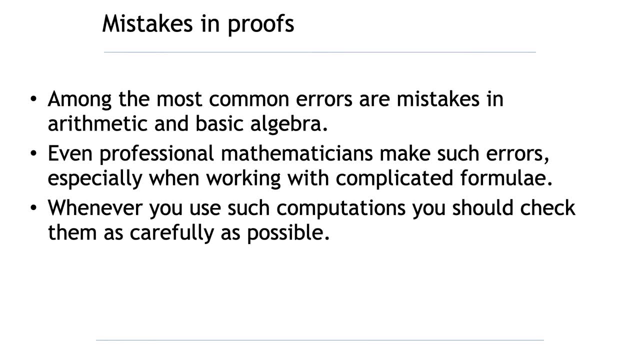 square of two integers is false using a counter example. Now let's see some mistakes that sometimes we can make when we are creating proofs. The most common errors are mistakes in arithmetic and basic algebra. Even professional mathematicians make such errors, especially when working with complicated formula. Whenever you use such computations, you should check them. 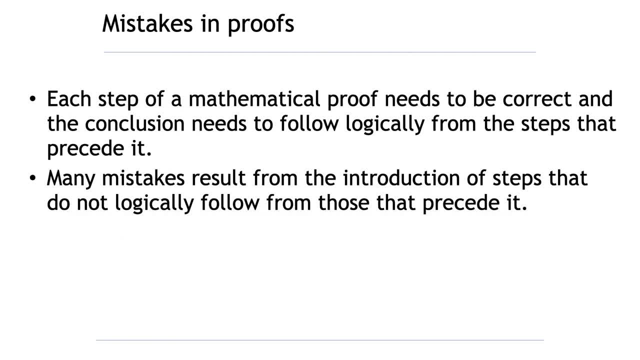 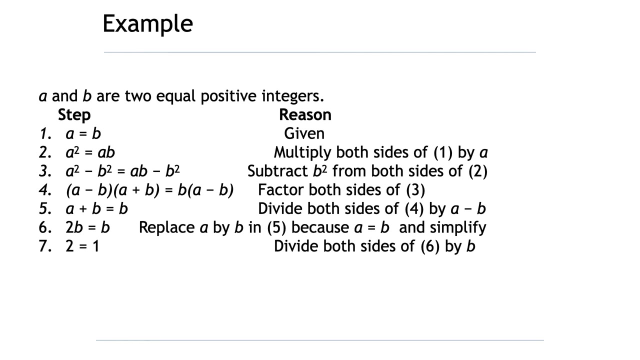 as carefully as possible. Each step of a mathematical proof needs to be corrected And the conclusion needs to follow logically from the steps that preceded. Many mistakes result from the introduction of steps that do not logically follow from those that preceded. Let's see this example. This is kind of a popular proof that you can find outside there. 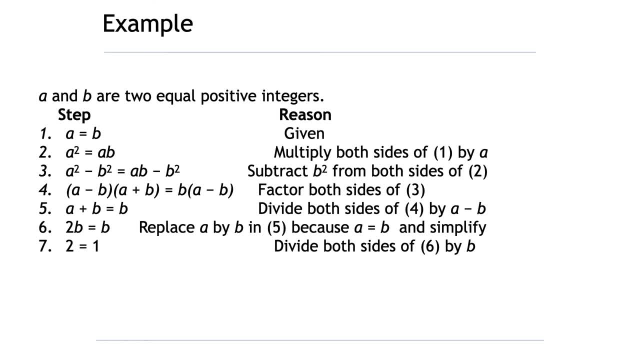 that it is a proof that two equals one. So let's see the steps. The premise of the theorem is: a and b are two equal positive integers, and from there someone is trying to draw the conclusion that two is equal to one. So the first step. 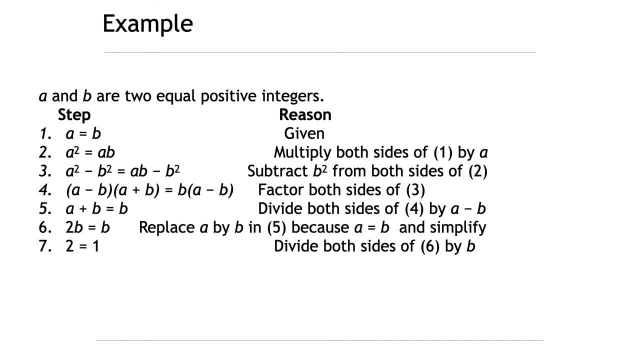 a equals b is given is the premise. Now, if we multiply both sides by a, we get a squared equal to ab. If we subtract b squared from both sides, then we get step three: a squared minus b squared equal to ab minus b squared. 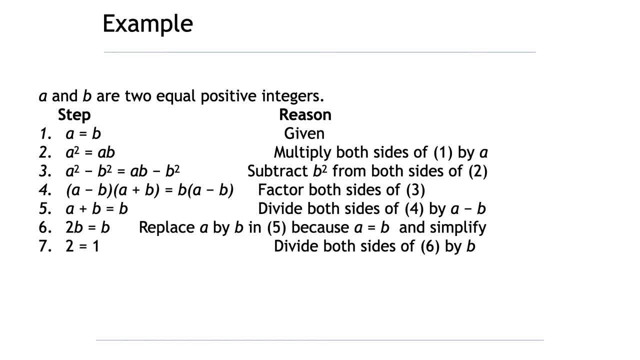 If we factor both sides, then we get a minus b. times a plus b equal to b. that multiplies a minus b. If we divide both sides of four of equation, four by a minus b, then we get a plus b is equal to b. After that, if we replace a by b, remember that a is equal to b. 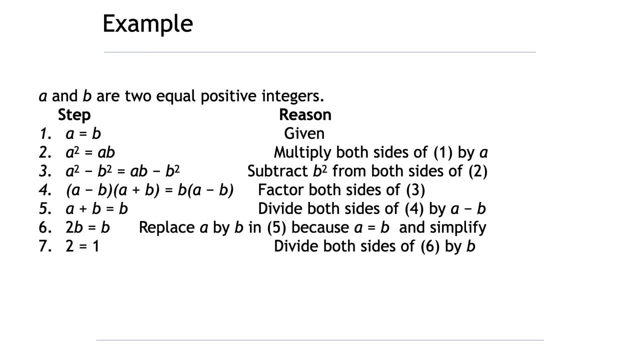 and simplify, we have that 2b equal to b. If we divide both sides by b, then we just apparently prove that 2 is equal to 1.. So everything looks good. What is where is the mistake here? The mistake is simple. The mistake we find it in step 5, when we divide both. 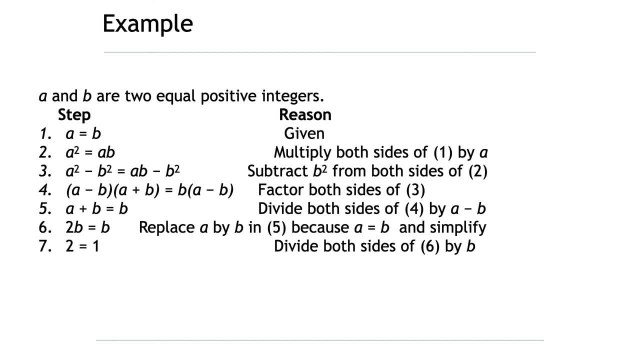 sides by a minus b. We cannot do that because a minus b is 0, because a and b are equal and, as you must know, division by 0 is undefined. so you cannot divide by a minus b because a minus b is equal to 0 and division by 0 is undefined. 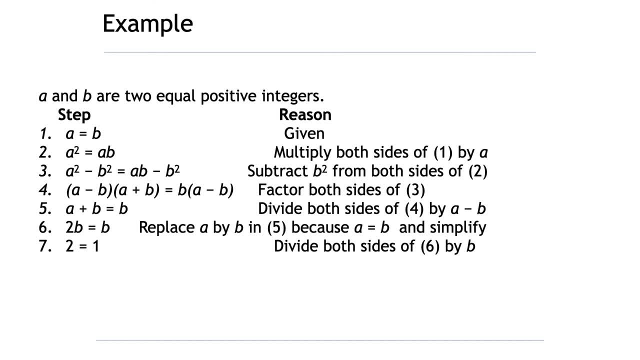 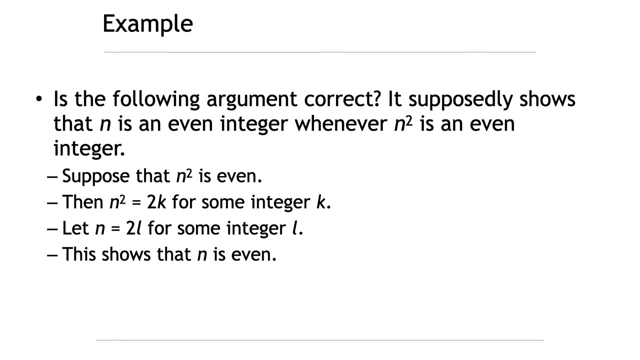 Here you just have a common error in this case for not to follow the rules of arithmetic. so you must be careful when you do proofs to not make a mistake on arithmetic or algebra. Let's see another example. Is the following argument correct? It supposedly shows that n is an even integer whenever n square is an even. 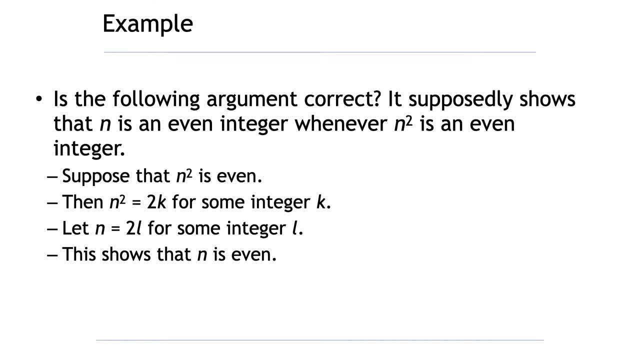 integer. Suppose that n squared is even then n squared is equal to 2k for some integer k. That's the definition. Now the next step: Let n equal to 2l for some integer l. This shows that n is even so. 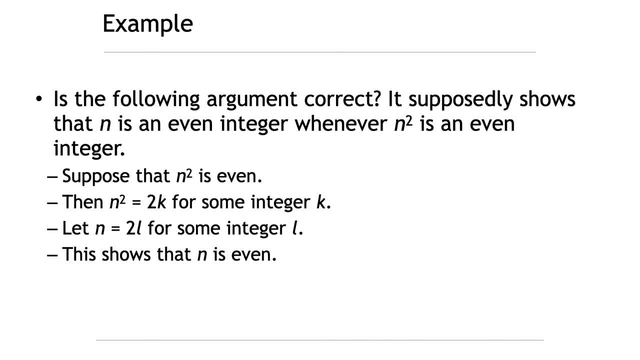 The argument is incorrect. We didn't give any argument to show that n can be written as 2 times l, for some integer l. As you can see, we are just assuming that n is equal to 2l. This is circular reasoning because we are assuming a. 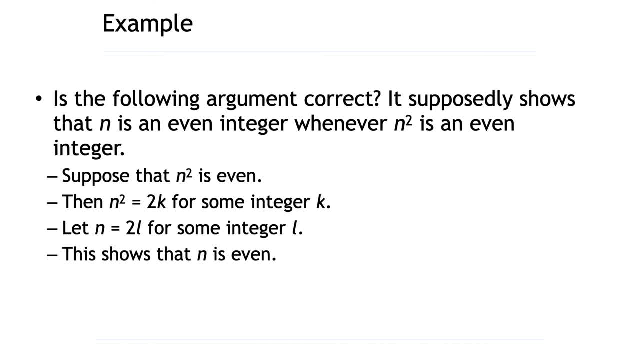 statement that is equivalent to the statement being proved In another way. you cannot assume a statement that is the same that you want to prove, okay, Otherwise the proof will never be right. Of course, the result itself is correct: n is an even integer whenever n, squared, is an even integer. What happened here is: 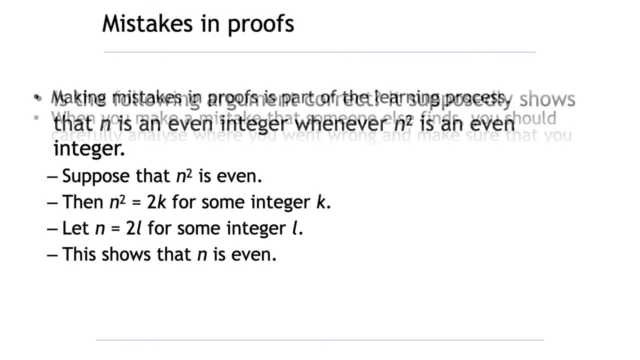 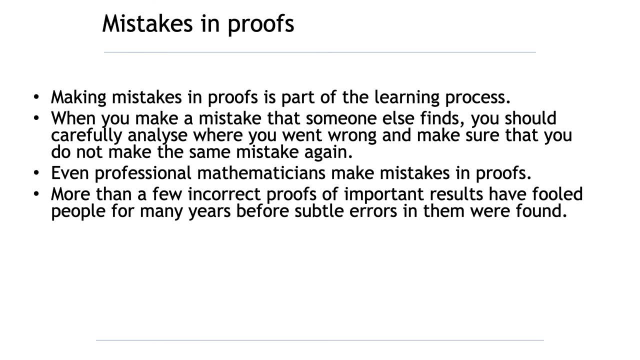 that the proof is the one that is wrong. Making mistakes in proofs is part of the learning process. When you make a mistake that someone else's someone else finds, you should carefully analyze where you went wrong and make sure that you do not make the 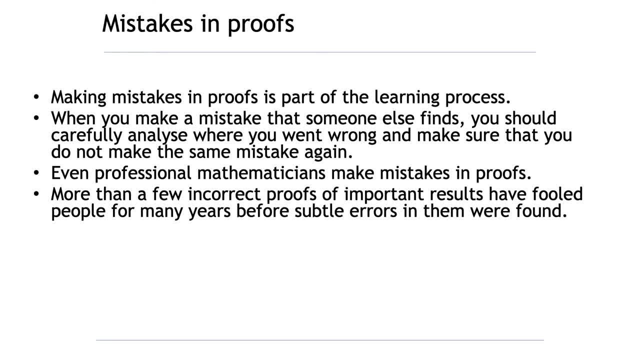 same mistake again. Even professional mathematicians make mistakes in proofs. More than a few incorrect proofs of important results have fooled people for many years before subtle errors in them were found. So don't be scared of making this type of mistakes. Remember, in this topic as in the rest of the topics in mathematics, the more you 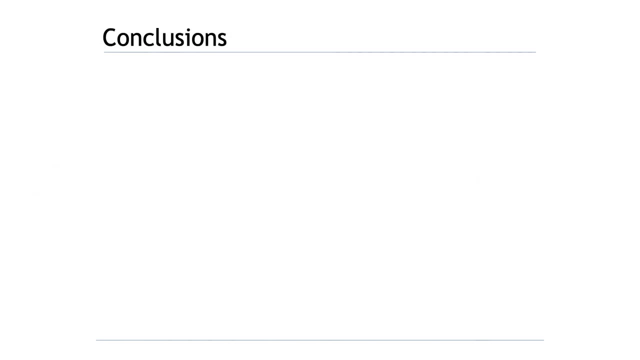 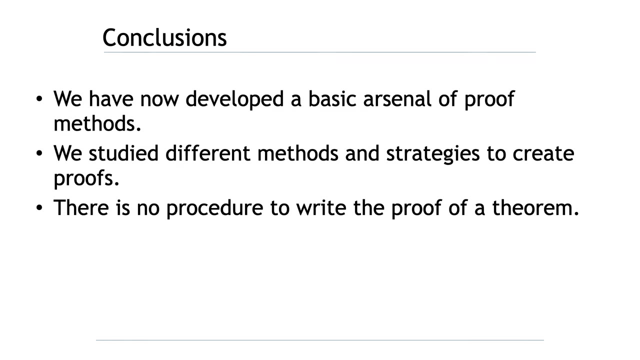 practice, the better you will get at it. So, as a conclusion, we have now developed a basic arsenal of proof methods. What we should do is we try one method. If we don't get the expected result, then we move to the next method in our arsenal. We study different methods and 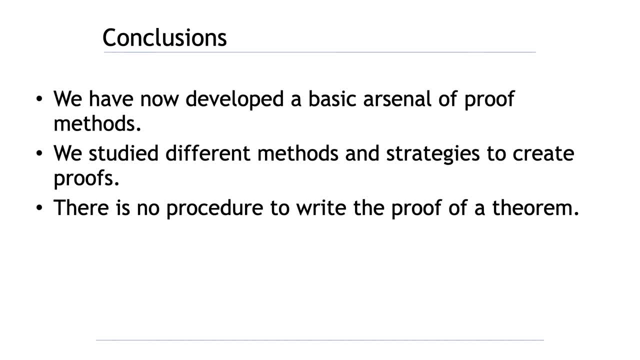 strategies to create proofs, And there is an important takeaway: that there is no procedure to write the proof of a theorem. You just use the general method and then you combine the axioms with rules and inference with premises on the best way you can. If you don't get the expected result, you try again using a.